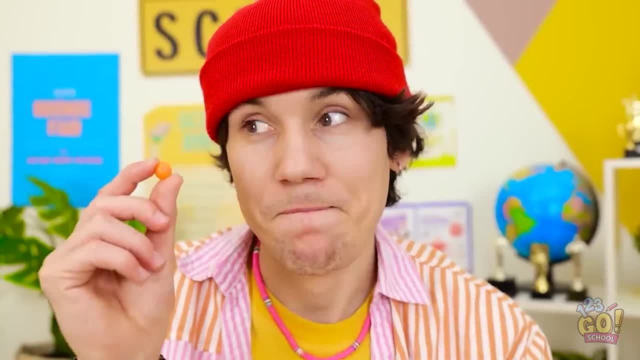 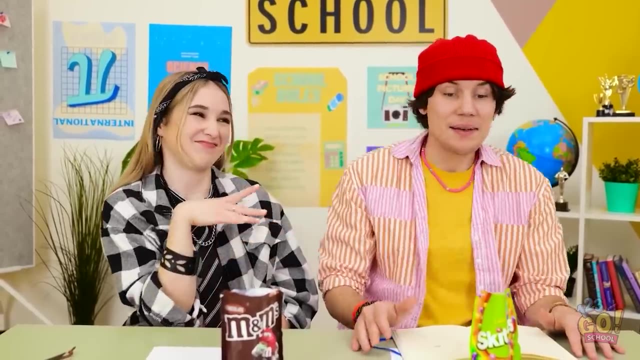 Please, I could do that with my eyes closed. Check this out, I'm about to blow your mind. Ugh My eye. What was that you were saying? Keep practicing, You'll get it eventually. Ahem, I want you to paint a rainbow, And it better be good. 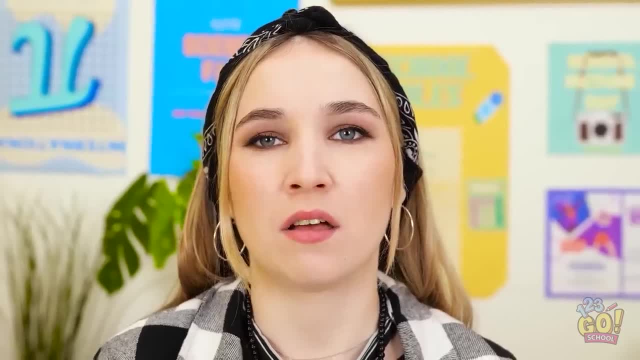 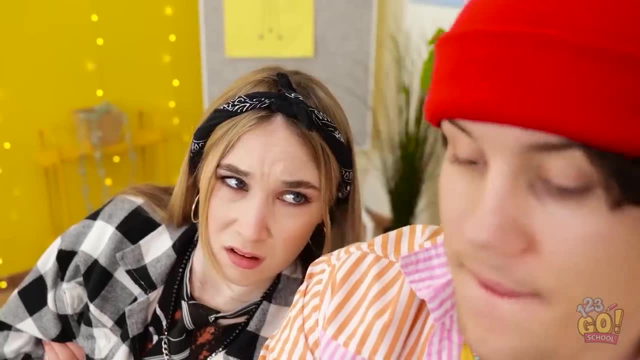 I love rainbows. I don't do colors. Who's laughing now? I can't wait to get started. There's just something magical about them. What are you doing? He's such a nerd, Annie. What are you waiting for? Get on with it. 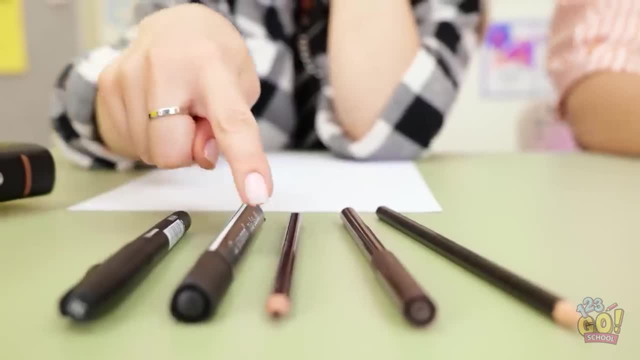 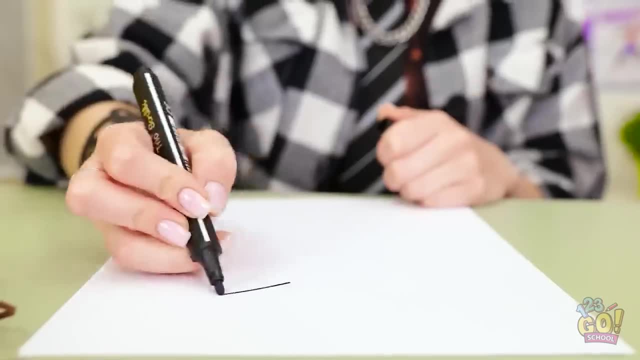 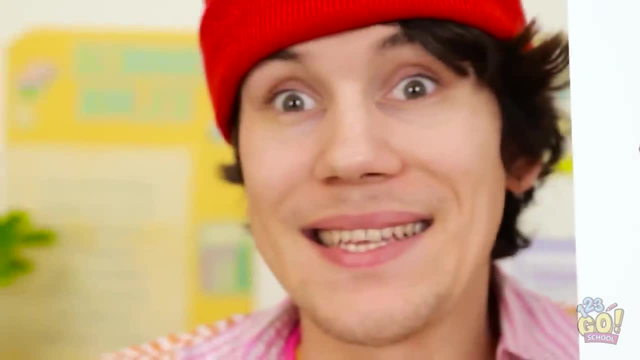 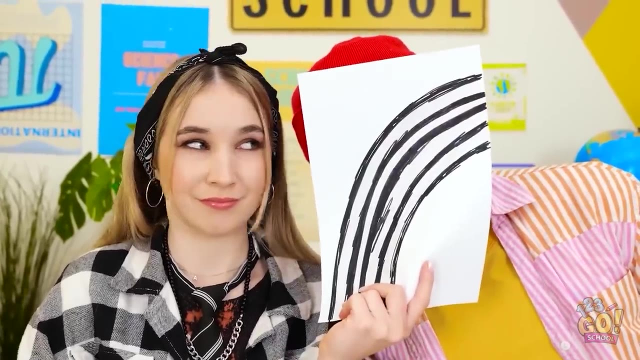 I finished. I wanted to capture the beauty of it. Do you like it? We've our very own Van Gogh-ing class. How's it going, Annie Ta-da, It's okay, You can hold the applause. You have seen a rainbow right. 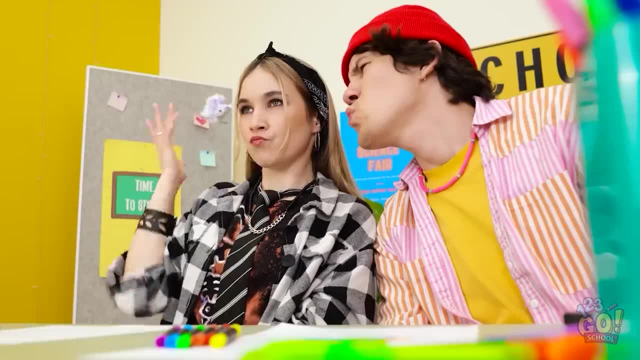 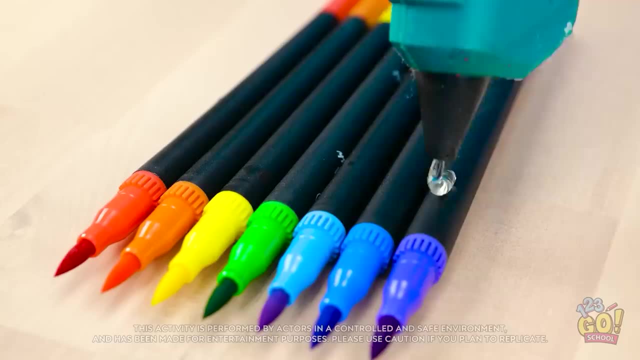 Ugh, This class is so stupid. This is what I think of your rainbow. Wait a second, Give me those pens. I'll arrange them in the order of… a rainbow. Then I'll need my glue gun. I'll glue the pens together. 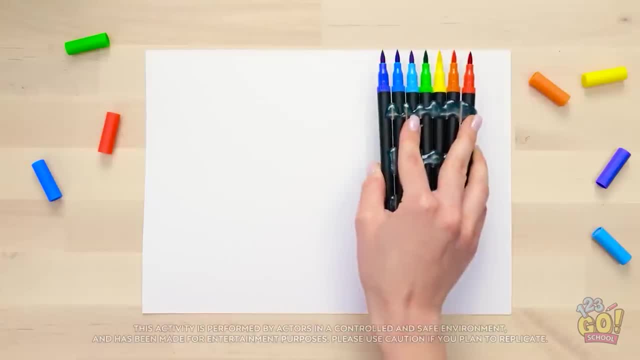 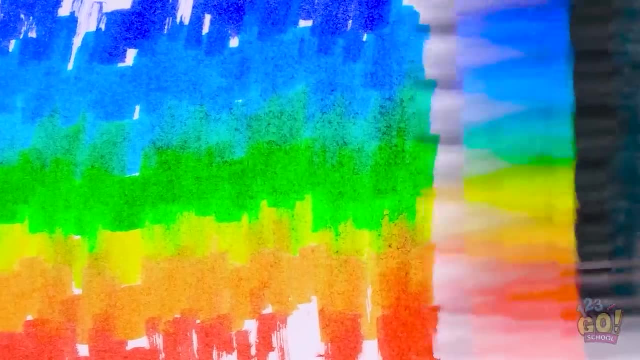 Then I'll wait for the glue to set. Now it's time to draw. I'll run the pens across the paper. I'll create an arc with them. Wow, This is looking good. The colors are blending together. This is such an easy way to draw. 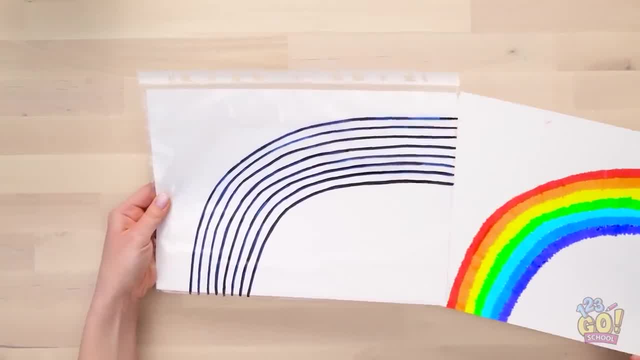 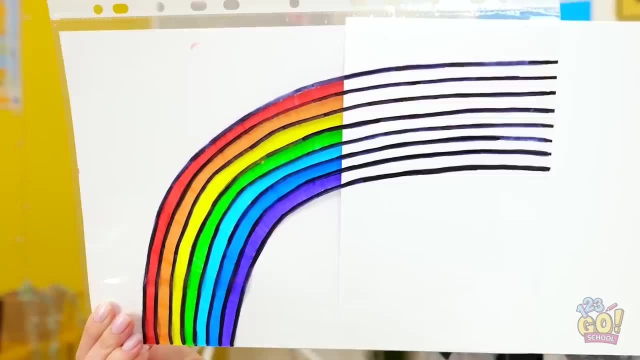 That's it, But I'm not done yet. I used a black pen to draw a rainbow on a plastic wallet. No, rainbow Rainbow. Pretty cool, huh. Now you see it, now you don't? Oh, And now I'm gonna draw a rainbow. 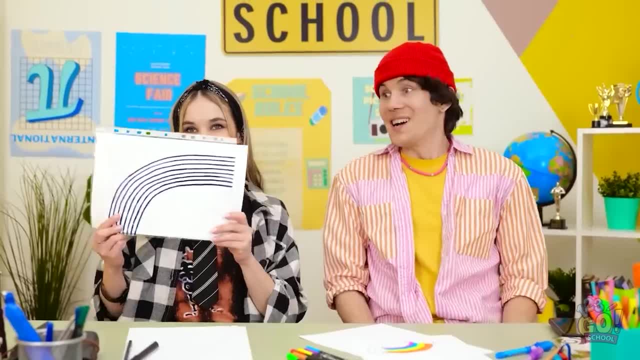 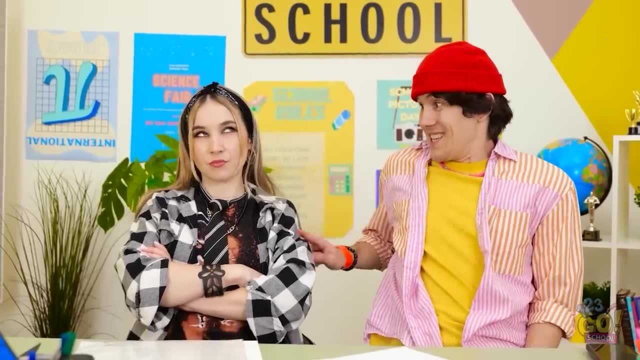 It's back again. What kind of sorcery is this? Wow, That's amazing. My work here is done. Wait a second, You have a multicolored t-shirt on. I thought you only liked black, What? No, You didn't see that. 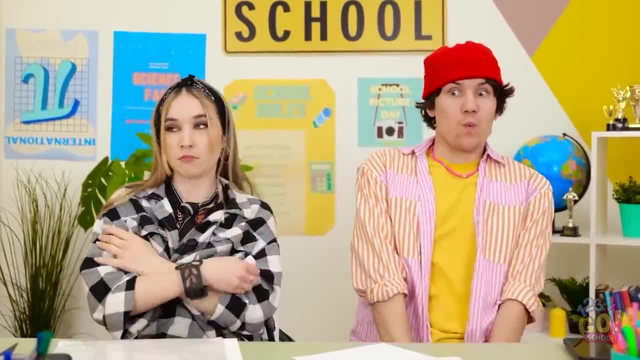 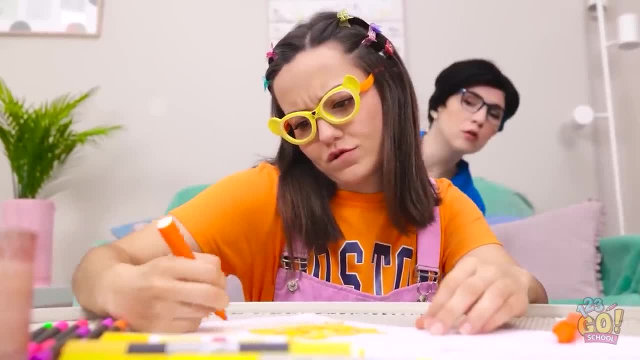 Don't say a word or else My lips are sealed. I've almost finished my homework. This drawing is gonna be great. Really, I wanna see. No, It's still a work in progress. Be patient, It's done and…it's beautiful. 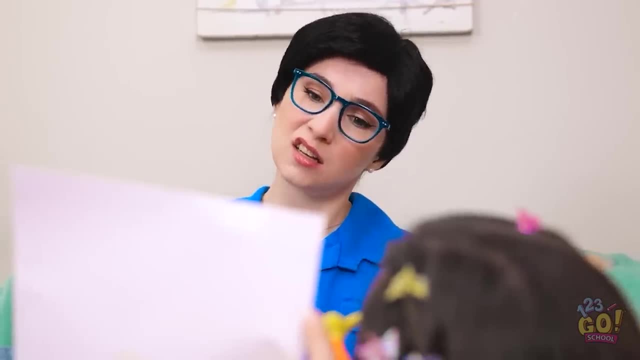 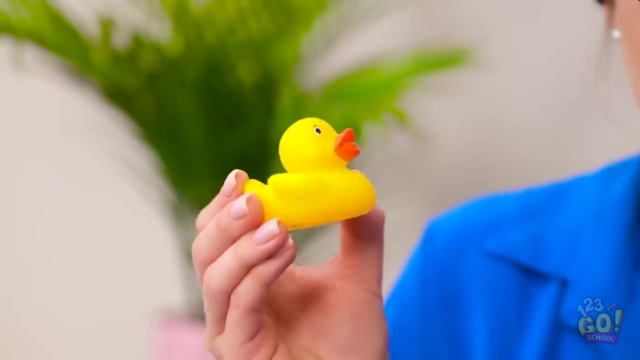 What do you think? Oh, It's uh…what is it? Is it a potato? Hold on, Maybe, if I squint. Oh, I see it now. It's a duck, What? No, I knew that I need a closer look. 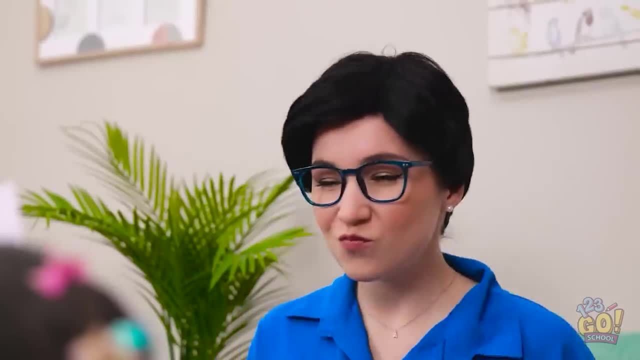 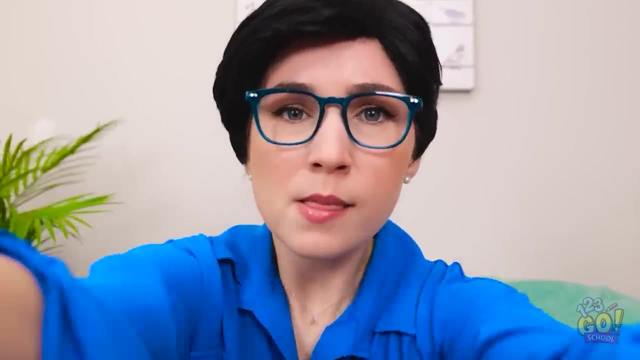 Like a really really close look. Ah, It's so obvious It's a lemon, isn't it? No, It's not a lemon, Right? I was afraid you'd say that. Hmm, This is tricky. What am I missing? 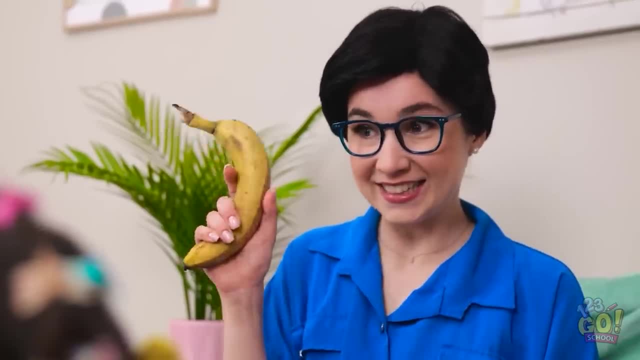 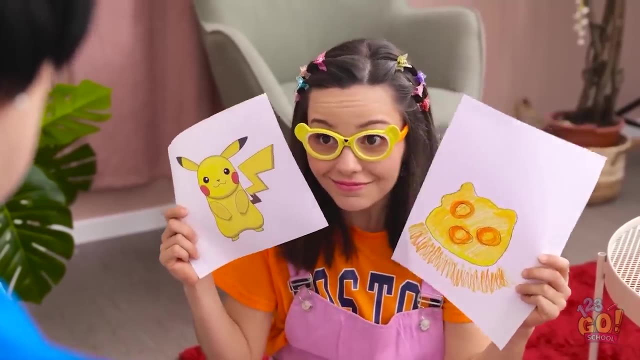 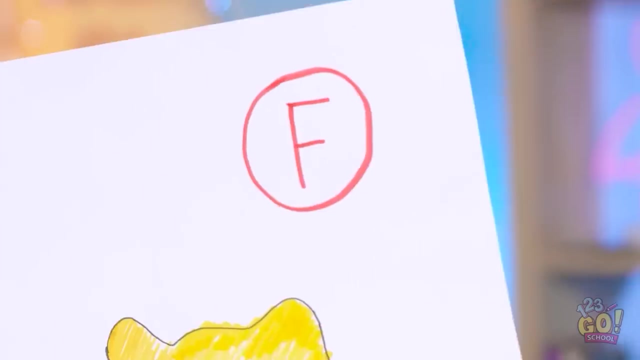 Are you kidding me? Of course, It's obviously a banana. You know, just forget it. I'm sorry, sweetie, What is it? It's Pikachu, Is it? This isn't good. Ooh, I wonder what grade I got. 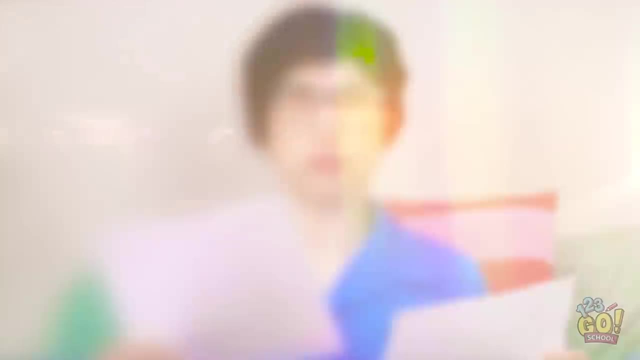 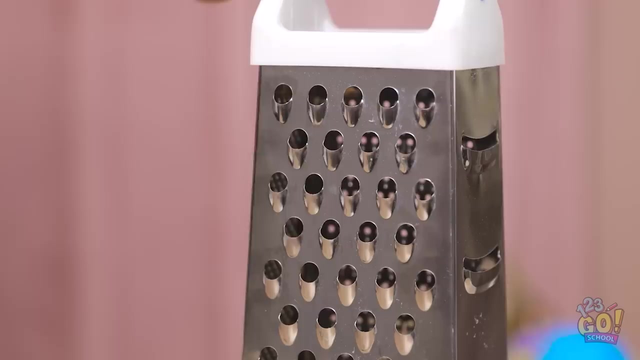 An F? Aww, This is the worst. She would be devastated, But I think I can fix this. I'll place Pikachu right here. Hmm, I'll need to sharpen this pencil. That reminds me I need to buy a pencil sharpener. 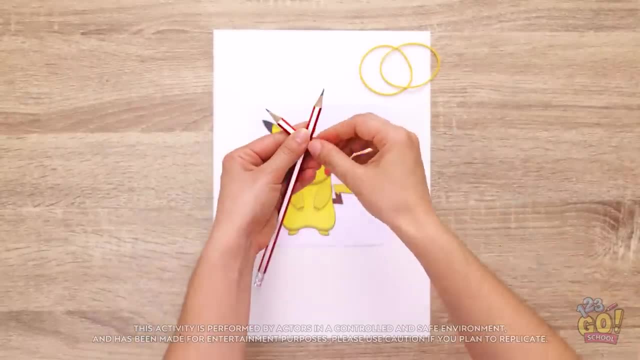 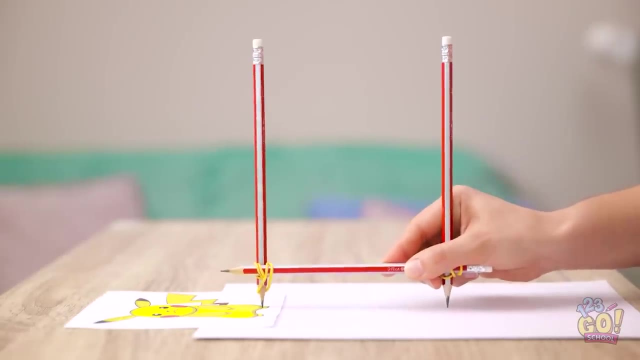 Ah, That's better. I'll take another pencil. Then I'll wrap a rubber band around them. I'll do the same at the other end. Now I'll draw around the image. I just need to follow the lines. The second pencil will trace it onto a blank piece of paper. 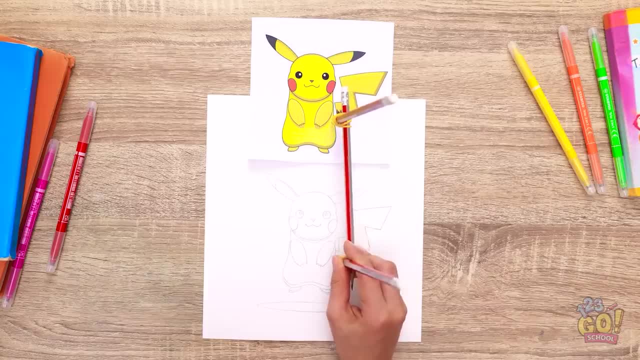 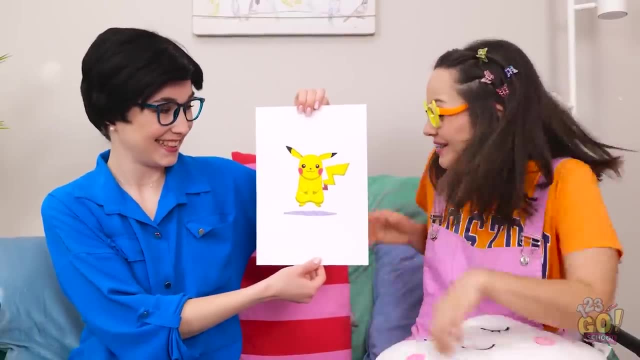 It's so much easier than drawing freehand There. It looks pretty good. I don't need this anymore. Now I need to add some color. What do you think, Ava? Wow, It's perfect. Thanks, Mom. I better get ready for school. 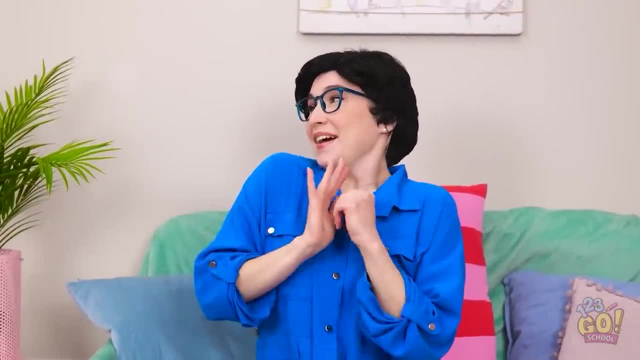 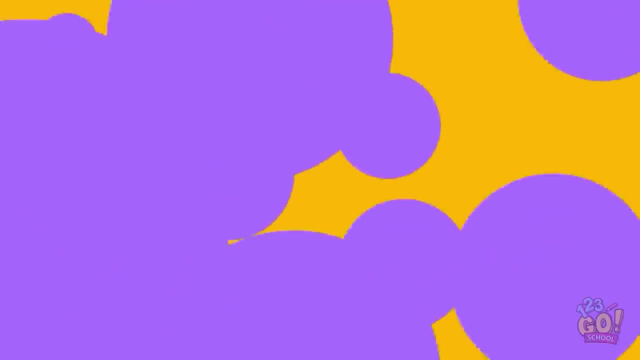 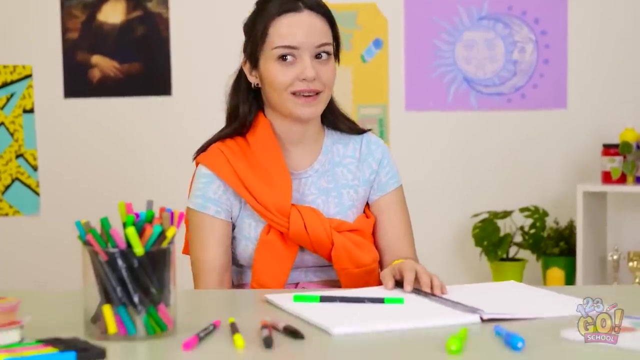 I don't want to be late. Have a good day, honey. Go get that A. Oh no, Ava, Wait, I'm so hungry, I need a snack. The teacher's busy. This is my chance. I always keep a snack under here in case of emergencies. 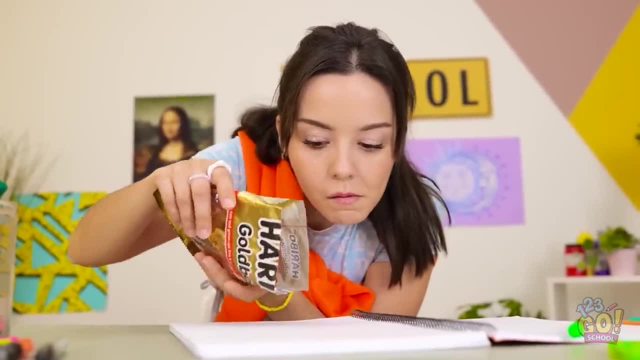 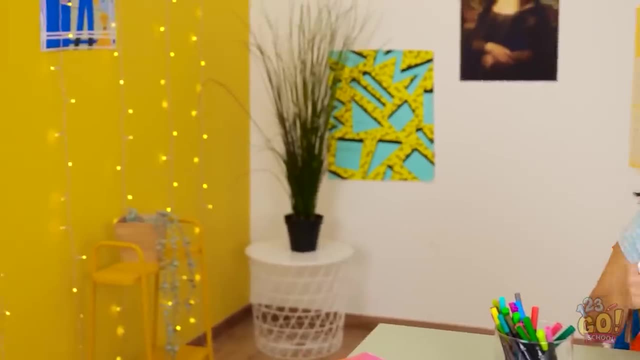 Ah, there it is. I'll need to be quick. She'll be so mad if she sees this. Was that candy? Hey, Uh, just ignore this. You didn't see a thing. What Don't you dare? You can't stop me. 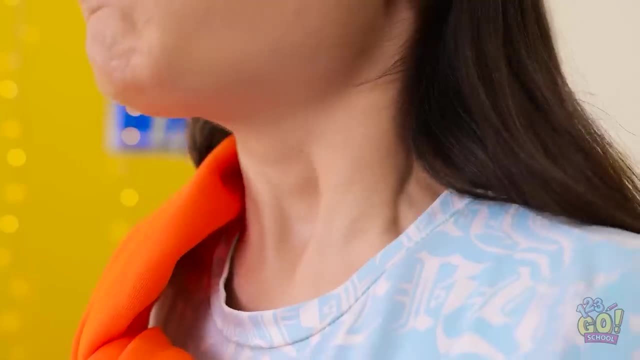 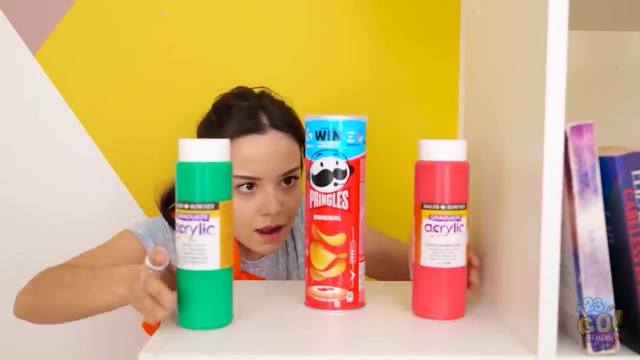 That's disgusting, Ava. I'm so ashamed of myself right now, But I don't regret it. I'm going to pretend that didn't happen. That didn't satisfy my snack attack. Luckily, I hid these chips. Mmm, These should do the trick. 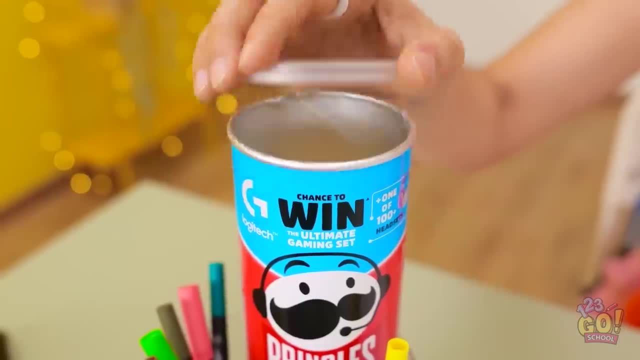 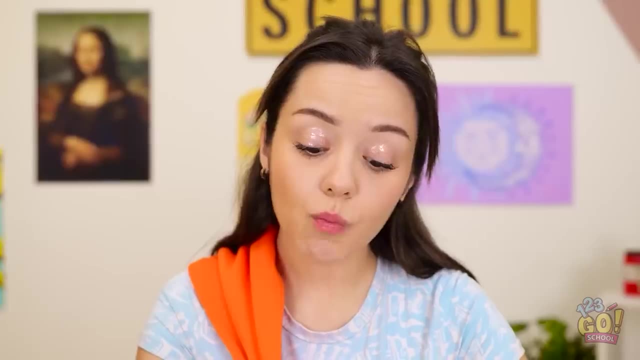 I'll need to hide them. Meh, My pencil holder will do. Just be cool. It's just another normal day. Mmm, That tastes so good. I needed that Open wide. Oh, that's kind of you. Wait a second. 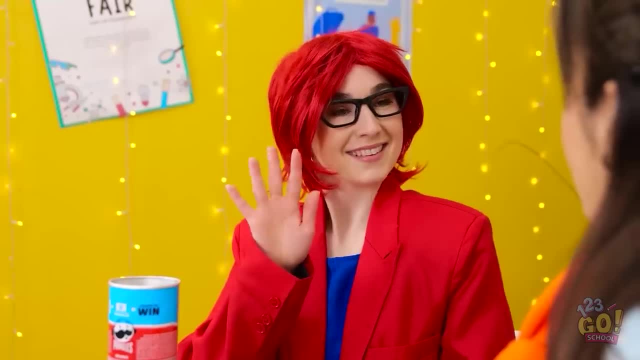 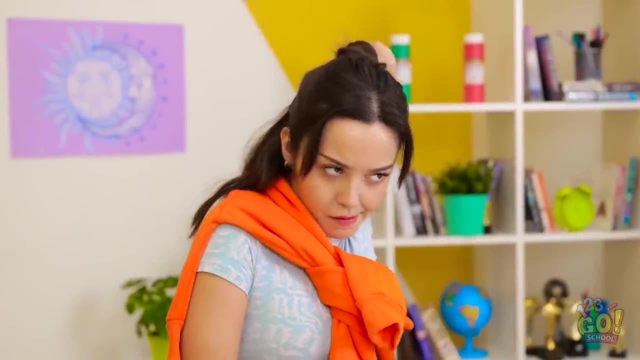 That's weird. I don't have a third hand. Hello Ava, No chips allowed. Do you hear me? Oh, I hear you, But you didn't say anything about donuts. What's going on Back there? Uh-oh, Divert, Divert. 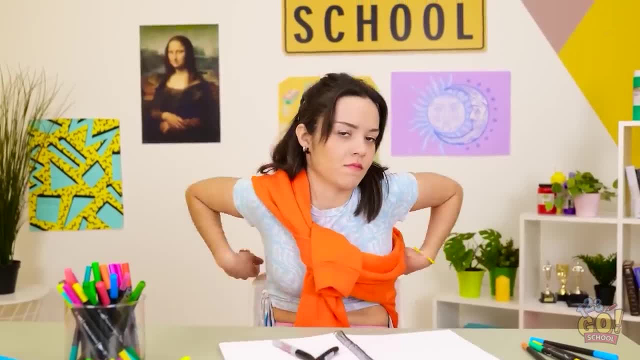 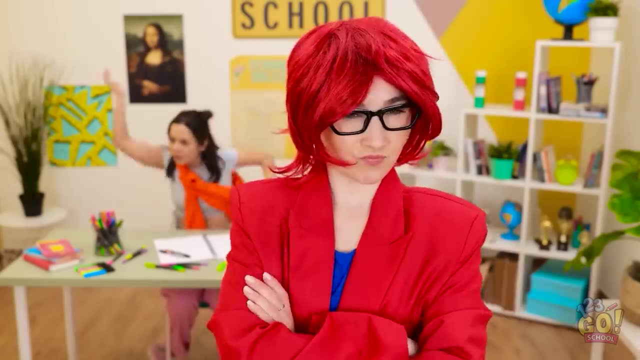 I'm watching you. Whatever, I'm too smart for her. Ha-ha, Gotcha What? Uh ooh, that's a bad itch. Something isn't right. She's a crafty one. This calls for some drastic action. 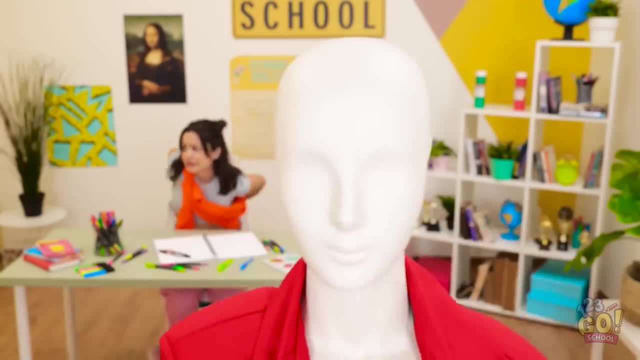 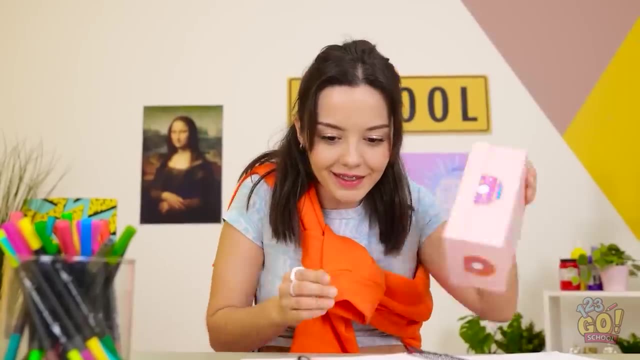 I knew this mannequin would come in handy. Now I need to give it a makeover. That's it. Keep looking away. That's what I'm looking for. I think I've earned this. It's the most delicious looking donut ever. 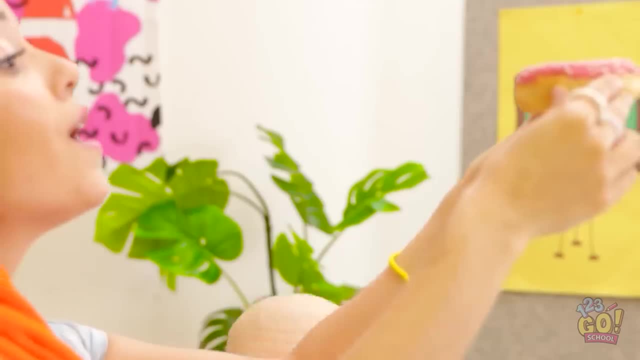 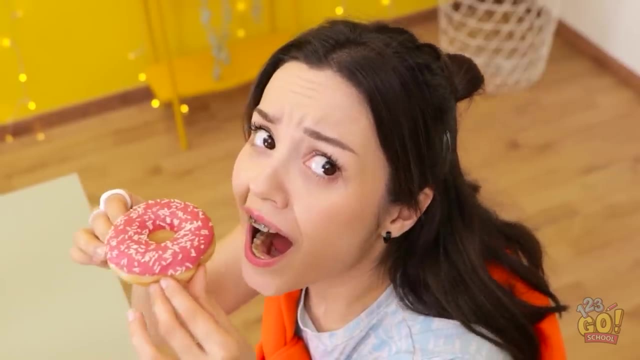 Pink frosting and sparkles. It's a work of art. Donut, eat that. I mean, do not eat that. I've warned you. Nooooo, Wait, you're bald Give me it. This is so unfair, You better not eat it. 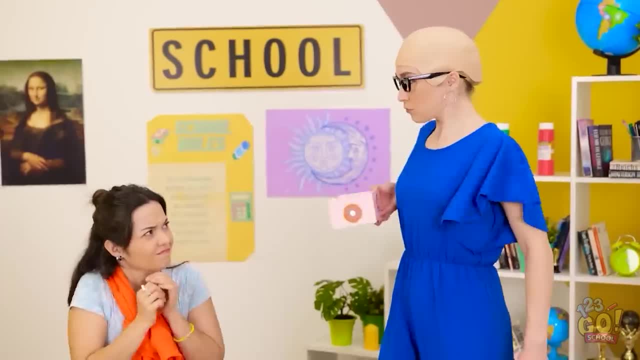 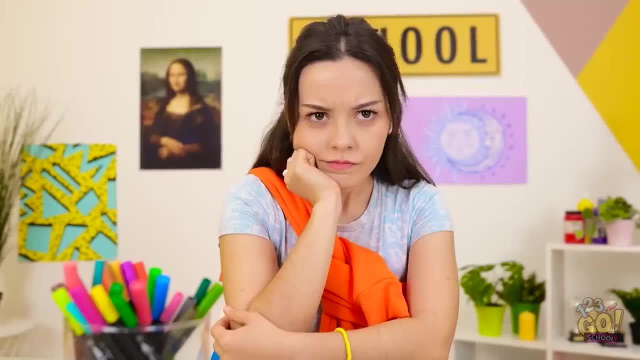 Let go Right now. Ava, If you only put this much effort into your schoolwork, No more got it. Now I have marking to do. Yes, fine, Wait a second. I have a great idea. I'll start by drawing two small circles. 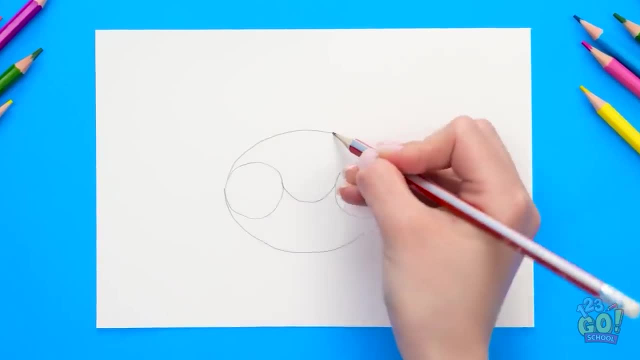 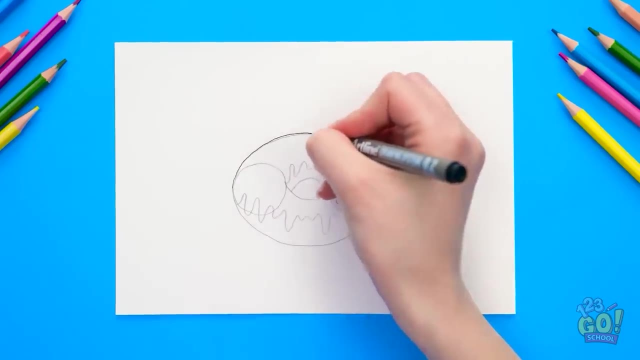 Then I'll join them up. I'll do the same on the top half. Next I'll draw a wave pattern. I'll do this all the way across, Then on the top half, Once I've sketched it in pencil, I can go over it with a pen. 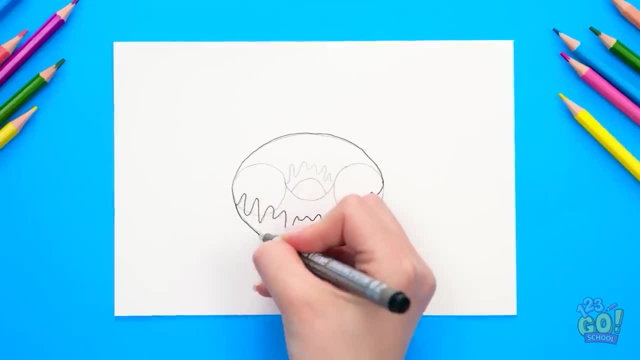 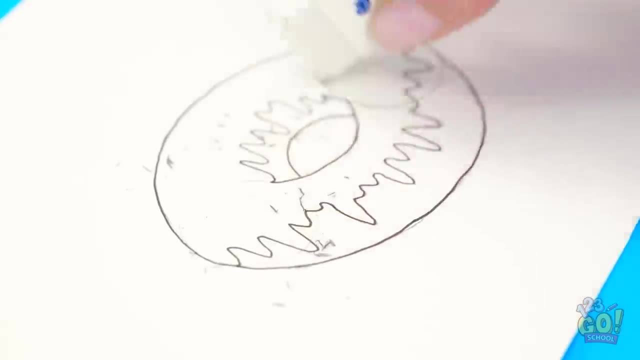 This'll make it stand out. It's just a case of following my rough drawing. I won't make any mistakes. It looks just like a donut. I can use an eraser to get rid of the pencil, Then I'll color it in. 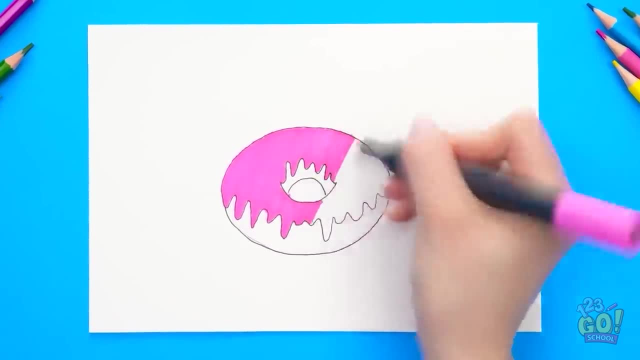 I'm only filling in the corners. I'm filling in the section inside the wavy line. This'll be the frosting. Mmm, my mouth is watering. Next, I can color the donut. I'm using a dark orange for this. 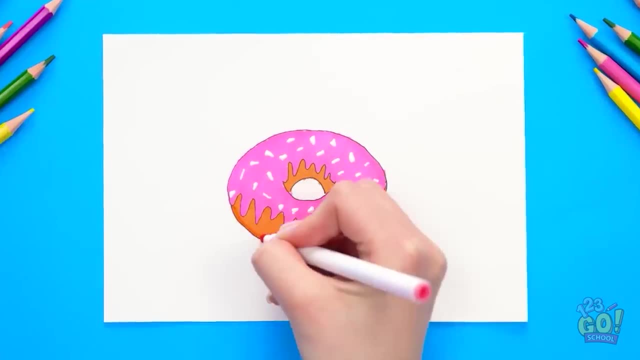 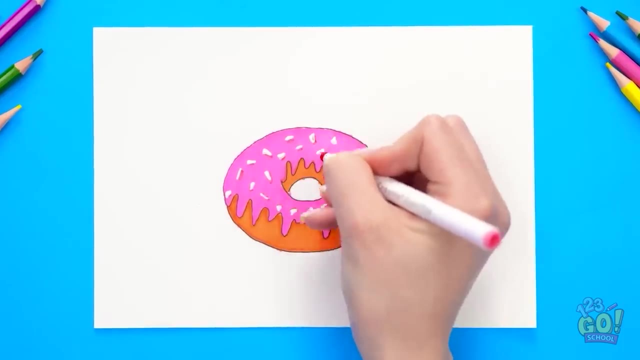 I'll use a correction pen for the sprinkles. I'll dab it over the frosting, Then I'll add some shadowing. It's just a case of going around the edges. I'll do the same with the sprinkles. It makes it look more realistic. 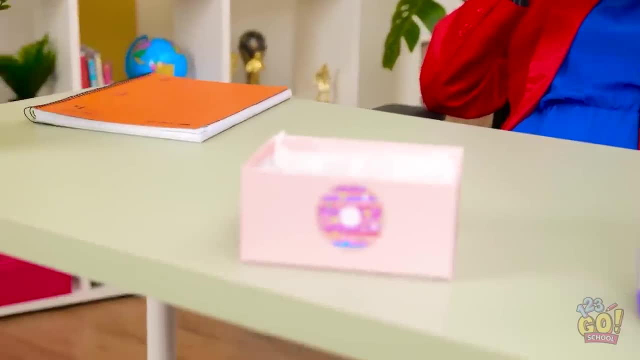 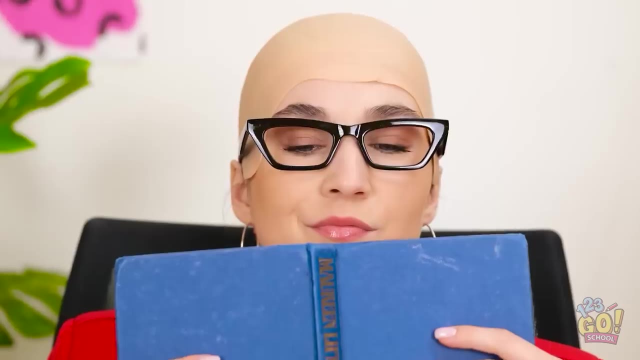 I think that's it Now for stage two. It's time for the ol' switcheroo. You're mine, donut, And I'll leave the drawing in the box. Huh, Who's that? I'm sure I heard something. 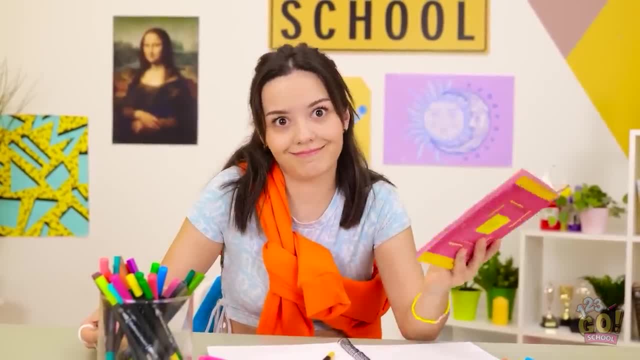 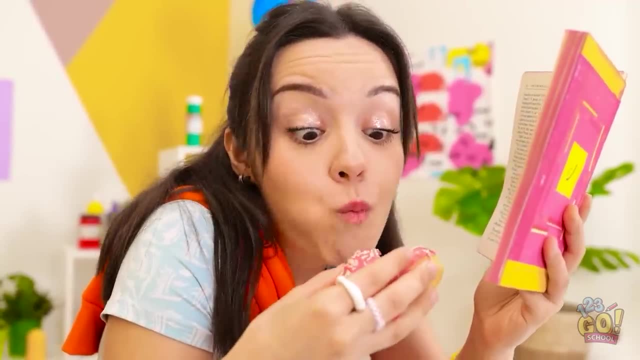 Hmm, What Is something wrong? I'm reading my book. Okay, but I'll be keeping my eye on you. Who knew books would be so useful? It's great for hiding my donut. Hurry along, Get to your next class. 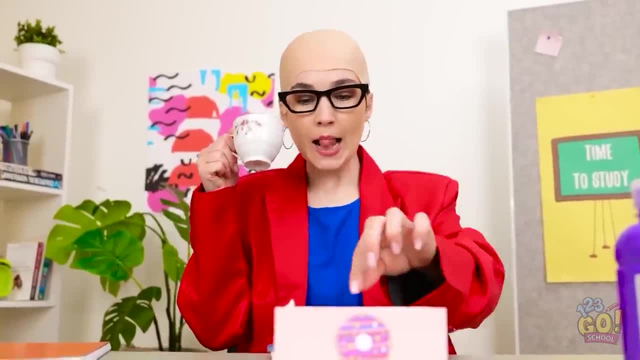 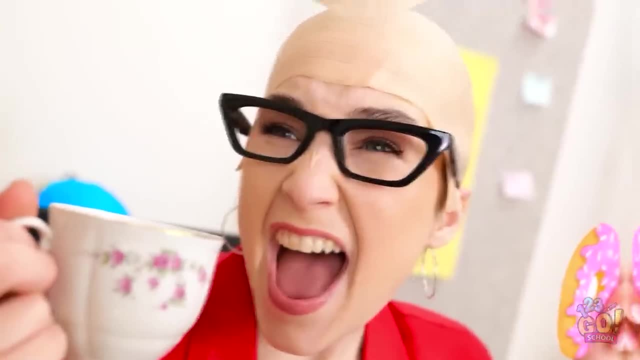 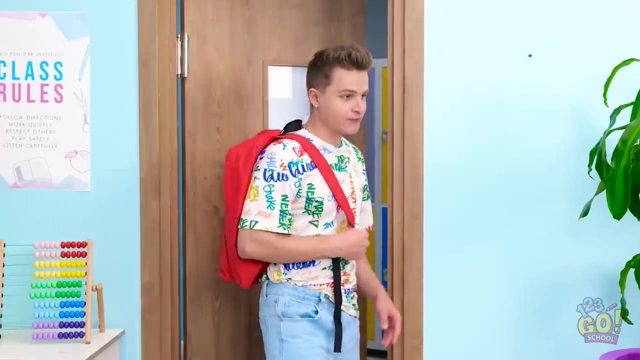 They're all gone at last. I've been looking forward to this. Wait, What's going on? This isn't a donut. I've been tricked. Avaaaaaaa Selfie That looks so cute. I hope I'm not late for class. 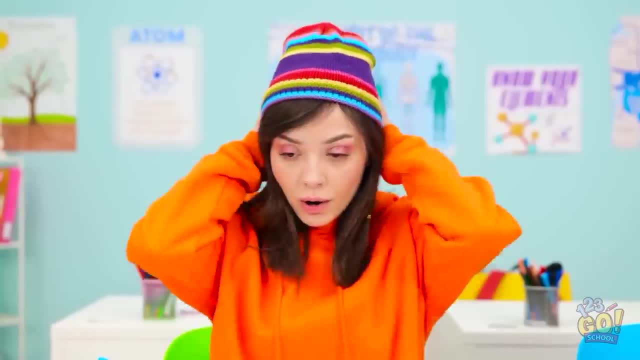 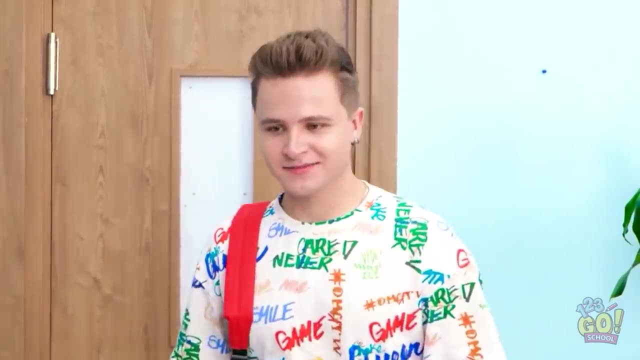 Uh, speaking of cute, check it out: it's Kevin. Oh my gosh, How do I look? Hey, Kevin, Over here. There you are. I was hoping to see you. Wow, he's so dreamy. We'd make a beautiful couple. 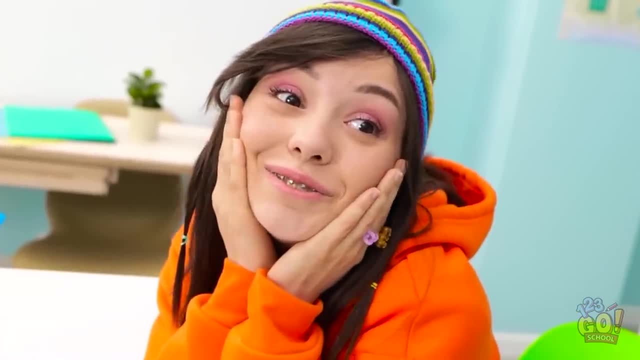 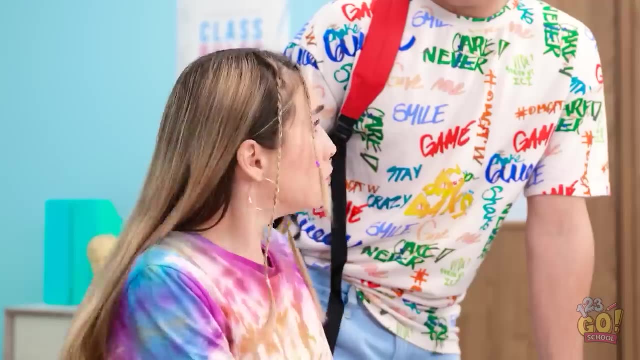 I wonder what our kids will be called. Who cares? they'd be adorable. Wait, What just happened? No, uh, it's not like that. You would say that I need to go, So I guess I'm alone again. 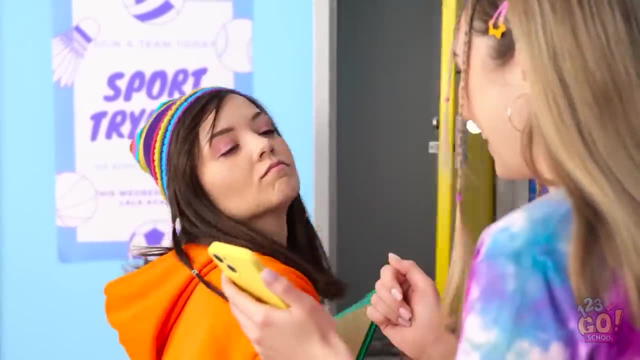 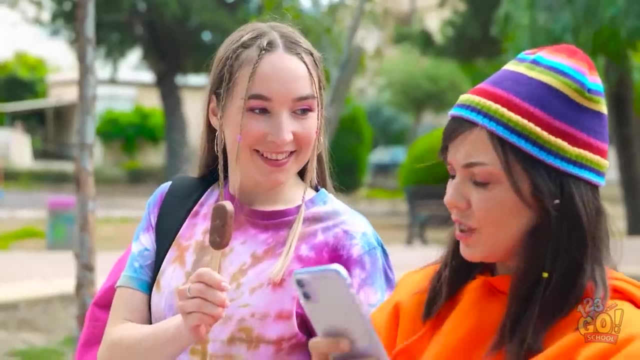 Hey, Ava, You need to see this. It's so funny, I don't think so. Uh, that was rude. Ava, There you are. I got you a popsicle. No, I don't want it. It's chocolate, Your favorite. 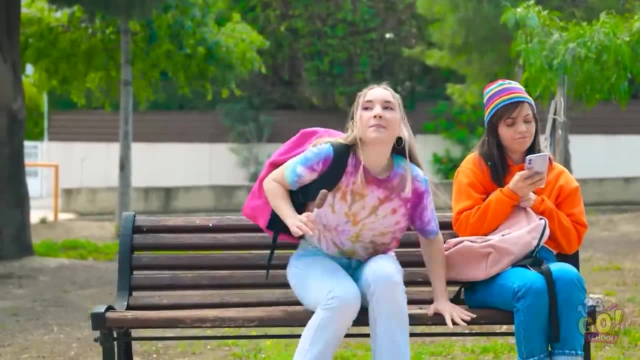 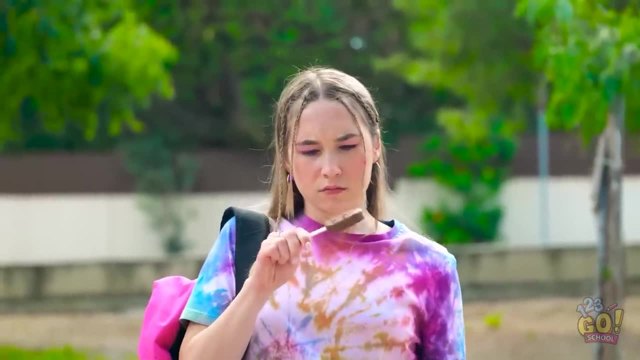 No, Go away, It's gonna melt. Okay, let's try this again About Kevin…. Oh, she's gone. Wait, Hmm, maybe I could use this. First, I need to cut out a circle from a piece of paper. 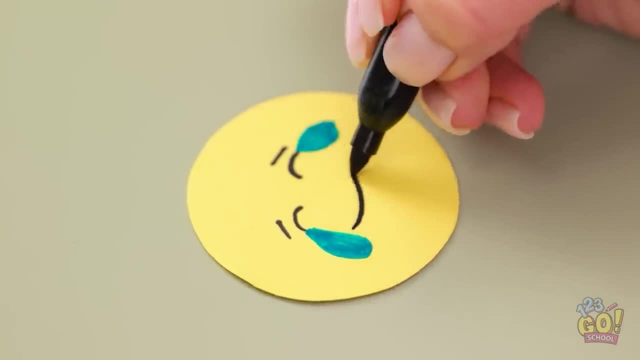 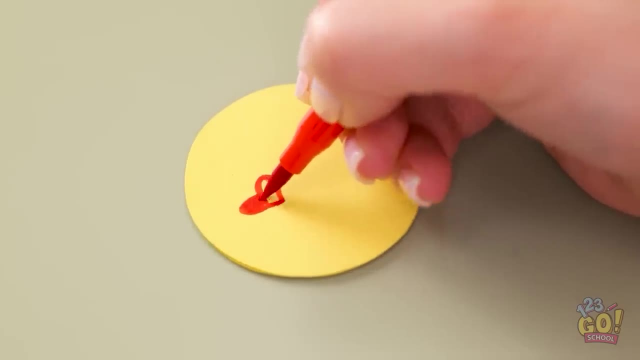 Then I'll draw a face on it. I think I'll go for the laughing crying emoji. It's a classic. Now I need a yellow and pink circle. I'll place them on top of the emoji. I'll decorate the top one with the love heart emoji. 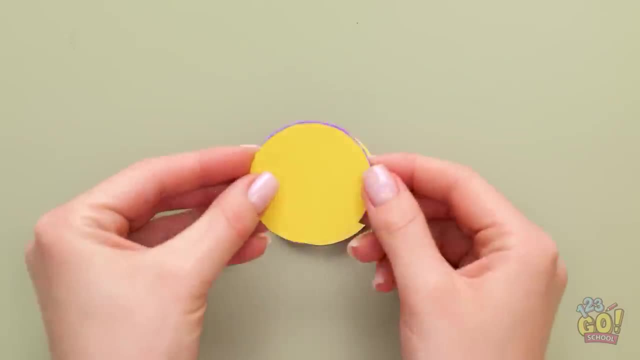 It's so cute. Just look at it. Then I'll add two more circles And draw another emoji. I think this one should be a sad face. Aw, cheer up, little guys. I'll put a pink circle on top of it. 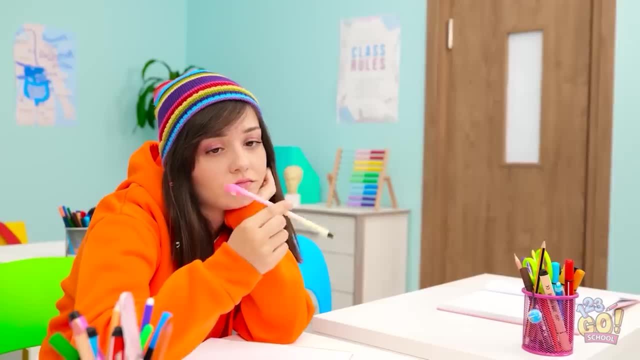 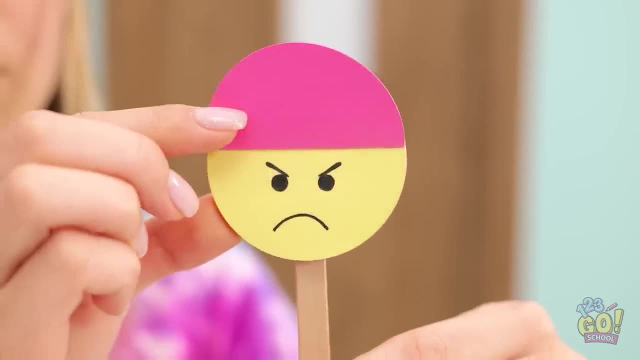 I'll flip it over and glue the popsicle stick to the back of it. I just want to be happy. Ava, you need to see this. What is it now? This is what you look like. We need to turn that frown upside down. 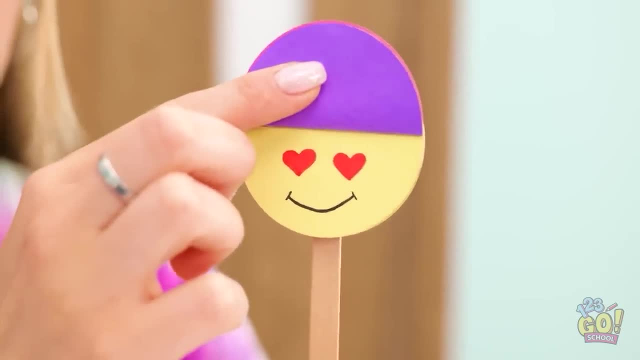 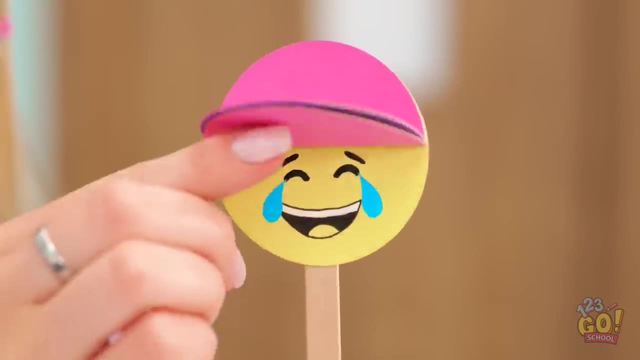 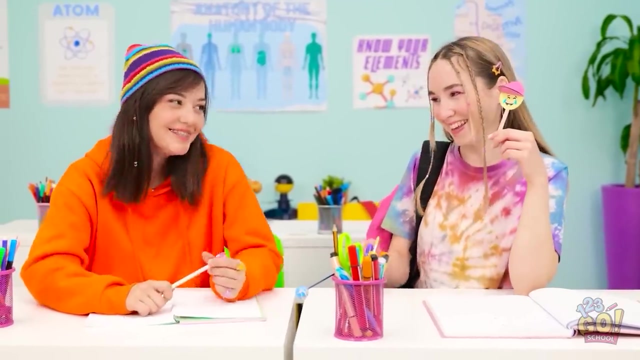 Very funny. This is how I feel. I love you. You're my bestie. You're so embarrassing. Yeah, I know, But it's funny, right, I suppose. so I'm sorry, Ava, I didn't mean for that to happen. 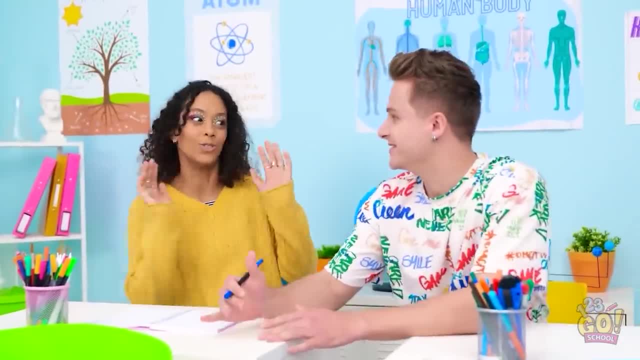 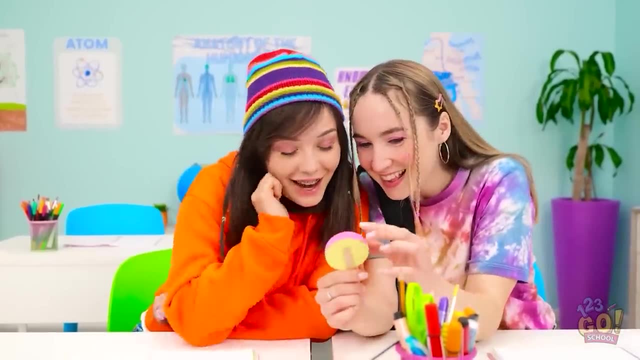 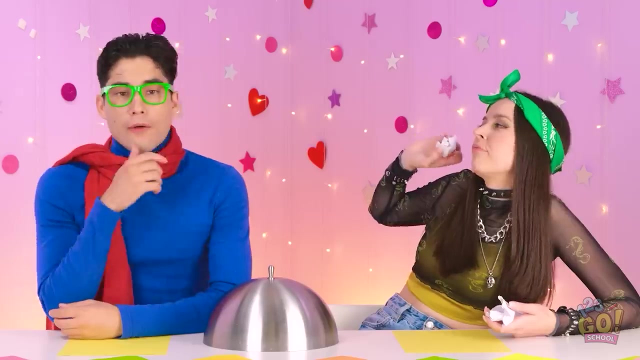 Hold on, Are you seeing this? No way, You're so funny, Kevin. Nah, he's not my type, So you made this. They live happily ever after. Do you mind? I'm listening to the story. You're such a nerd. 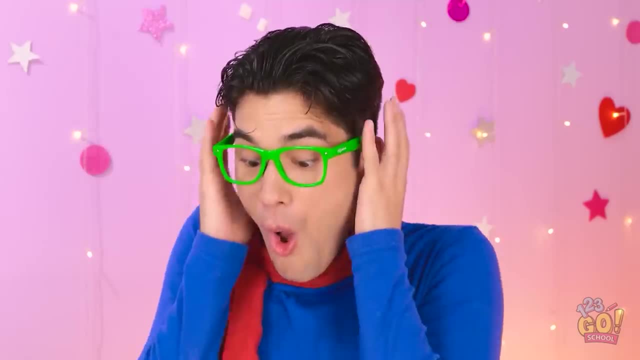 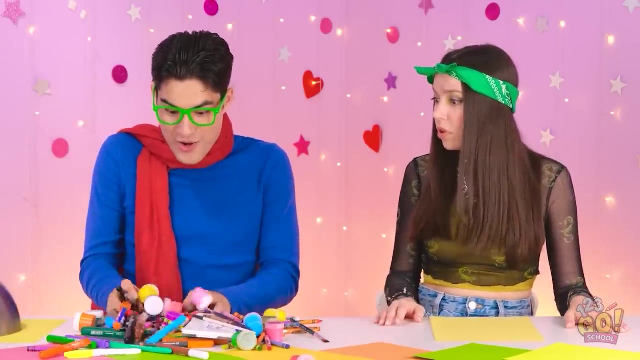 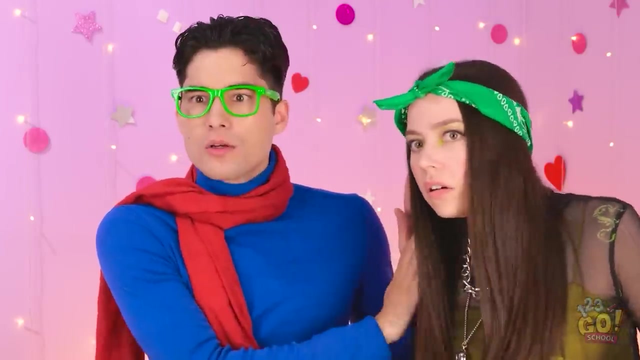 Luna, Stop hitting the nerd, Bring on the supplies. Whoa, Is this for me? So where's mine? Whoa, Look at all these art supplies. Are you kidding me? This is awesome. Uh, do you mind You'll need a model? 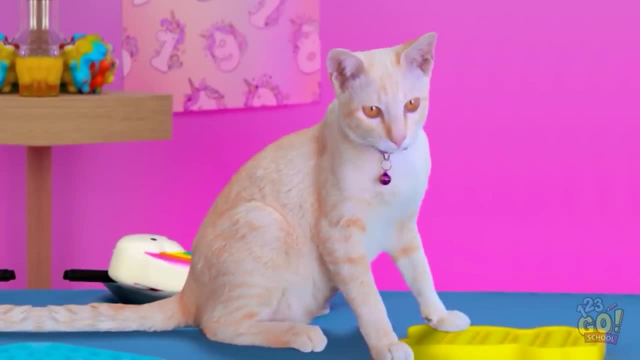 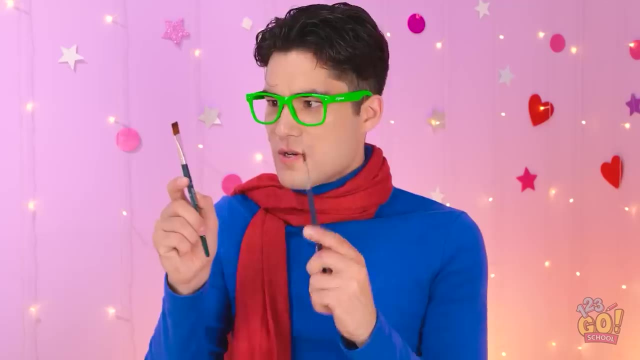 This cute little cat will do. It's purr-fect, Haha. Awww, It's so adorable. I'm ready to create. Hmm, Which brush, though? I need something to draw with. These crayons are perfect. 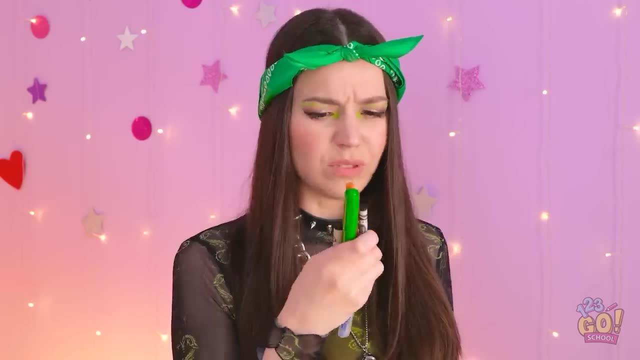 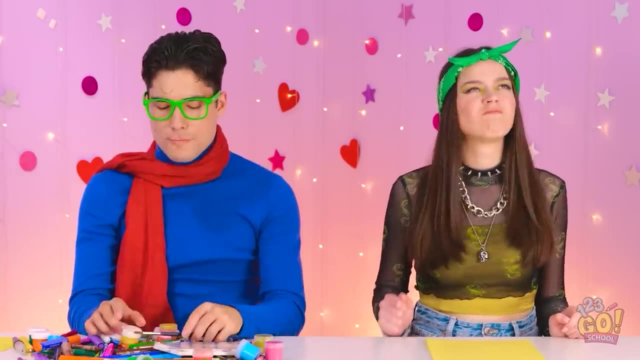 Nope, No way Put them back. We're gonna have a problem. Maybe I should use pens instead. There's too many choices. This is so annoying. Wait, I have an idea. I just need to be sneaky Just a little further. 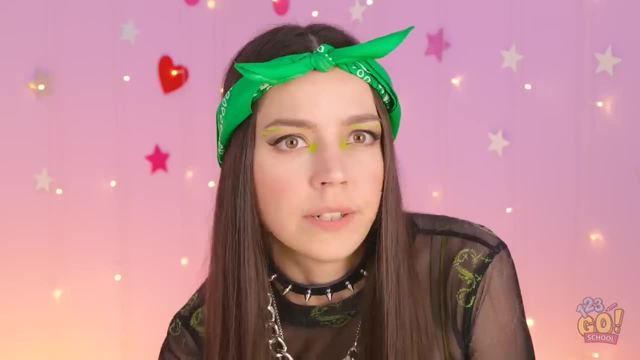 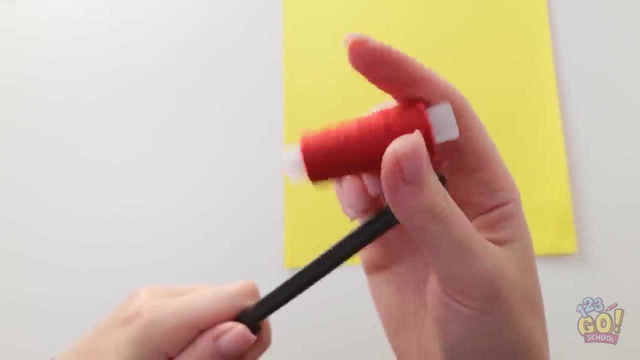 Huh, Just that cool. Now's my chance. Got him. Hah, You're not so smart after all. What am I supposed to do with these? At least I've got a pen. I better get started First. I'll draw a straight line. 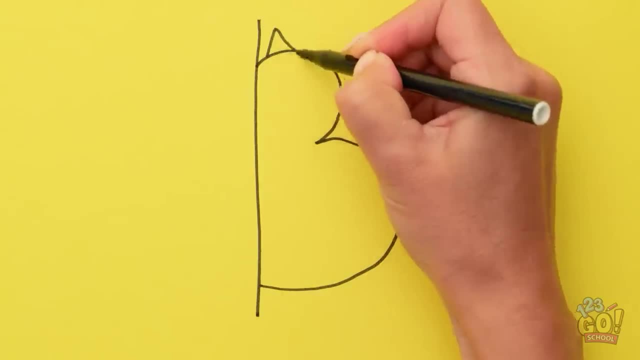 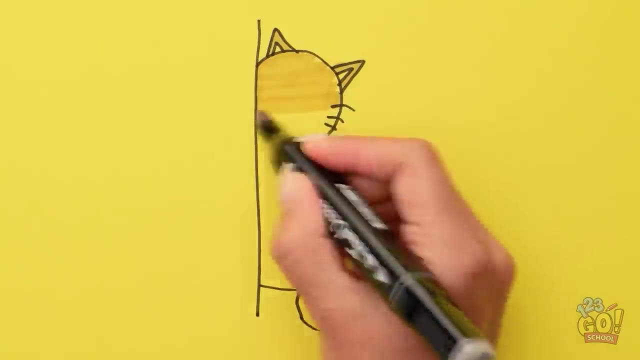 Then I'll draw a large number three, Just like this. Next I'll do the cat's ears And some whiskers. Finally, a long curvy tail. Let's add some color. This is looking good. It's time to add the eyes and nose. 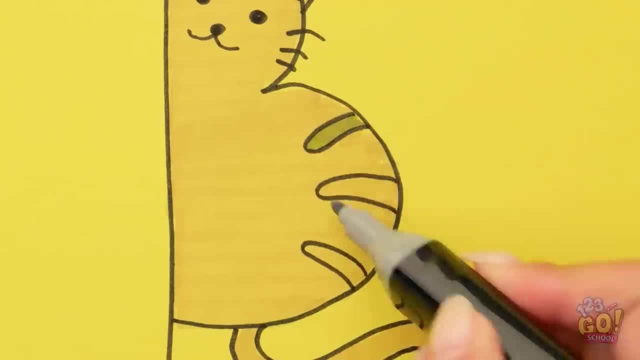 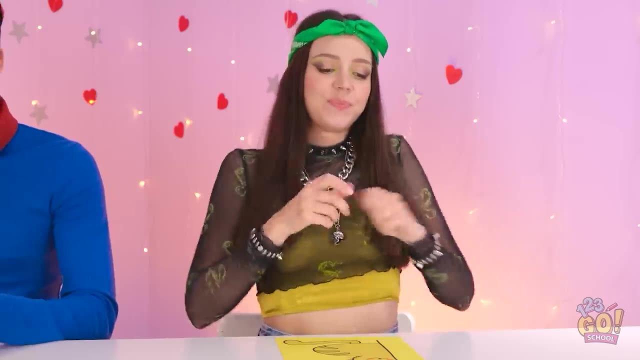 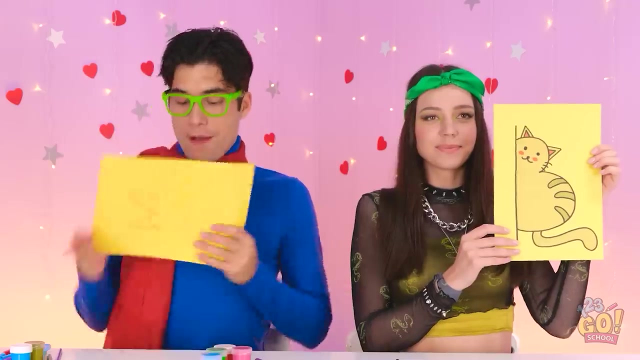 I'll give my cat some stripes. I'll make these darker. It needs some rosy red cheeks. Pretty cute. huh, That was easy. Hey, You know I finished right. Oh no, I'm not good under pressure, I need to be quick. 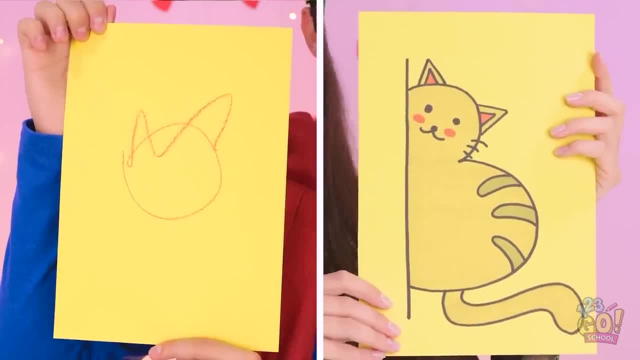 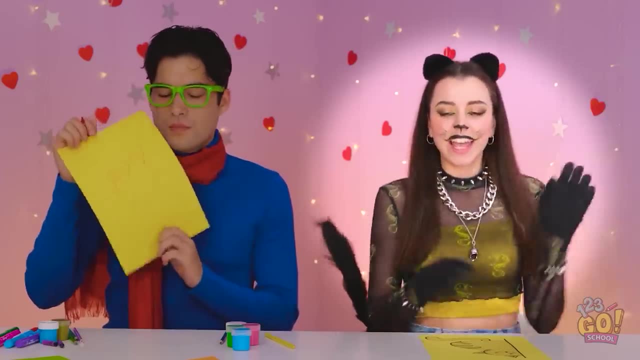 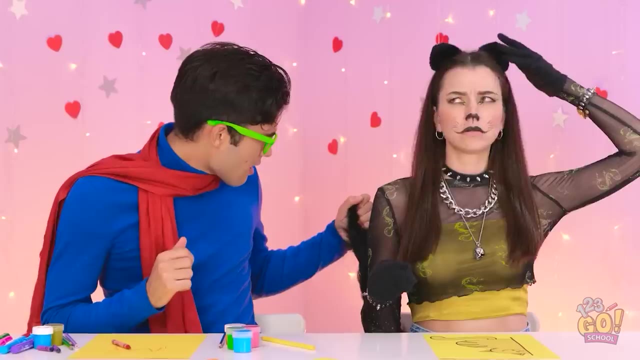 Tada, There's an obvious winner. I'm the judge And the winner is… LUNA. Yes, I knew it. Woohoo, Hey, what do I win? Wait, something's different… Wow, look at this. 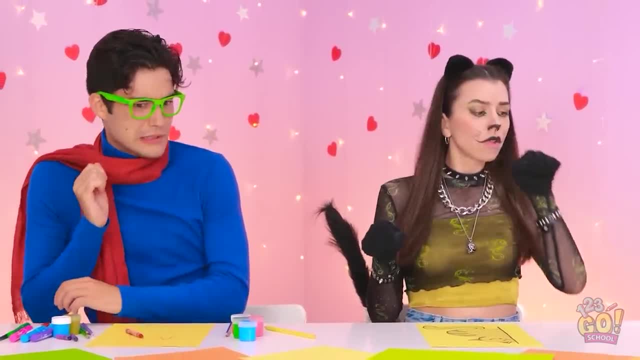 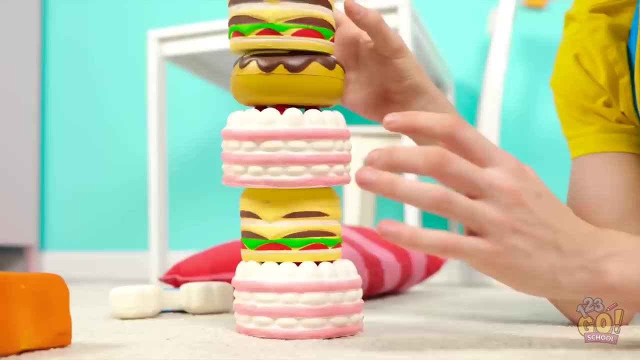 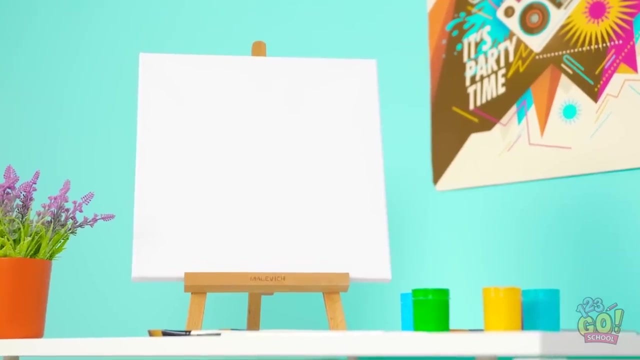 Get your hands off my tail. You're a mean kitty. No wonder I'm a dog person. Almost done stacking my foods. No, It's falling Shoot, I'm so bad at this. Wait, is that paint up there? Yeah, It is paint And an easel. 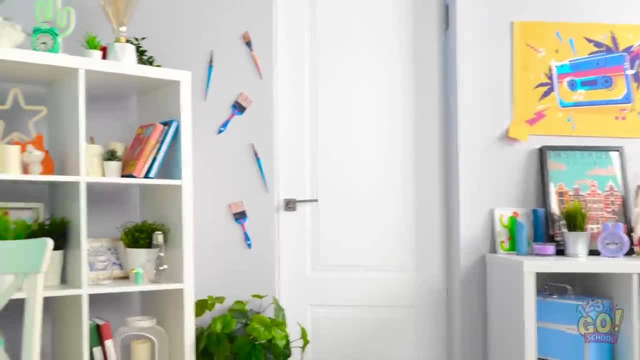 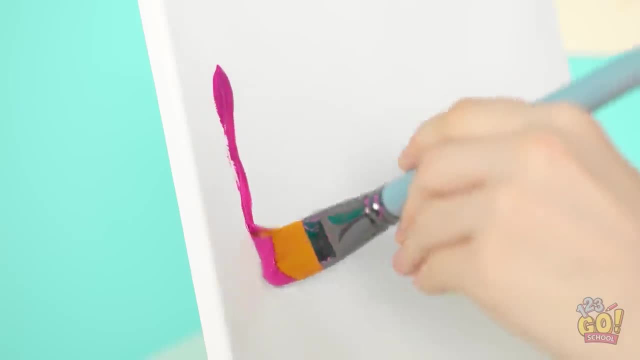 She left them out. I'm gonna do some art. Is she around? I don't want to get caught. Nope, The door's shut Time for painting. I like this pink color. It's pretty. I'm so good at painting- The best even. 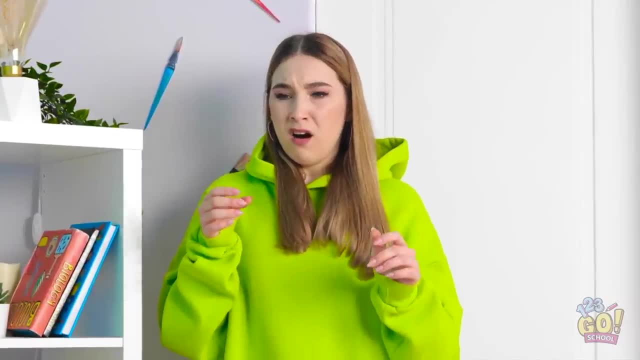 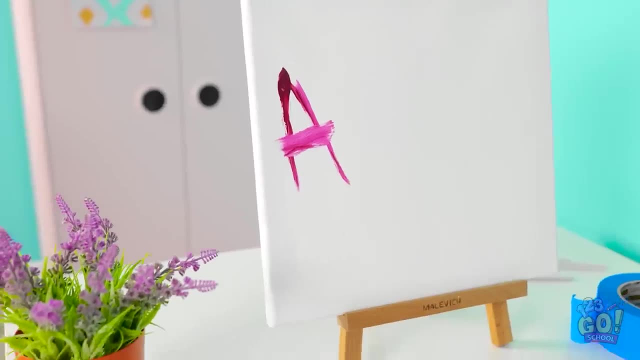 All right, Got the supplies I need. What The Heck? Hi, Look I'm painting, Isn't it good? Um sure, I guess. so What am I gonna do? He's already ruined the canvas. Yes, 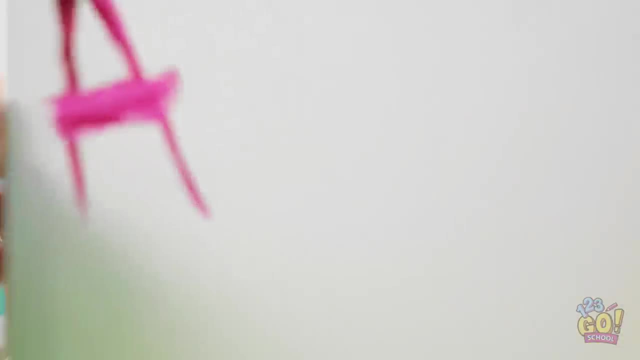 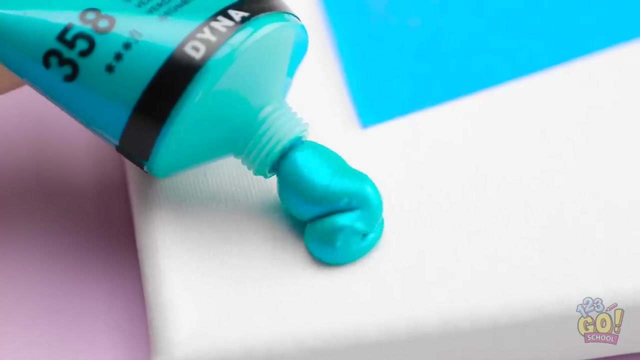 I think I've got a solution. All right, I've got the canvas. A perfect A Time for some paint. I'll use the color he used- Blue over here. I need more blue and some yellow- All the colors. Time to do some cleaning with the sponge. 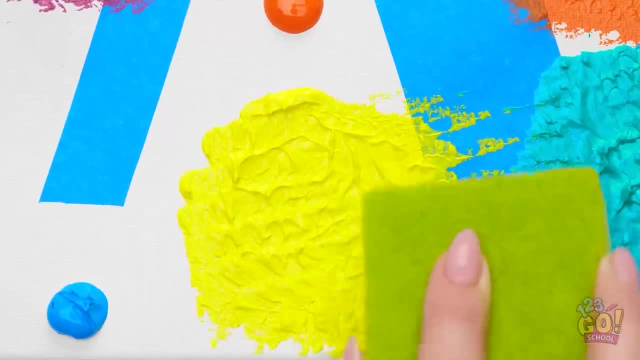 Just kidding. This is part of the art. I want to use the sponge to dab at all the paint colors. It's okay if I get some on the tape Turns out, doing this dabbing is a good idea. It's pretty fun. 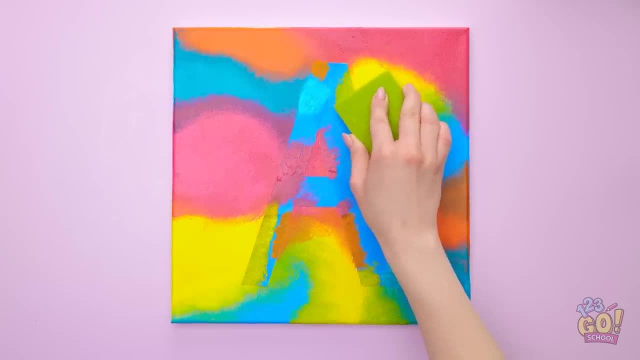 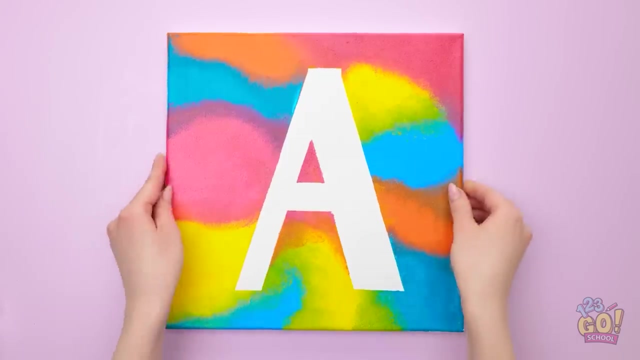 But it's not really all that quick, Not if you want to do it well, anyway, Phew, There we go. I finally covered the canvas with all the paint. Here I go, Pulling off the tape. It comes right off. 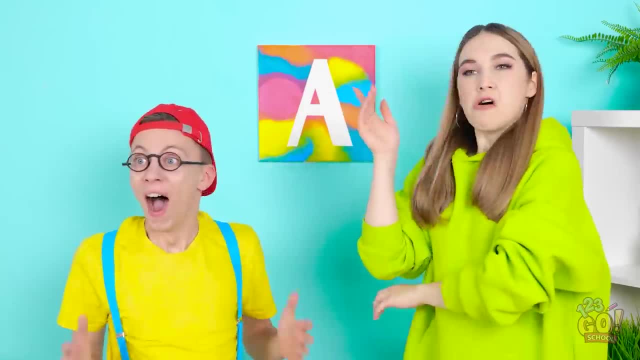 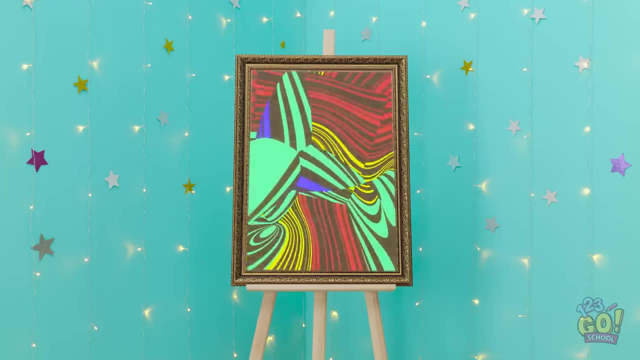 Wow, It looks amazing. It turned out great. Wow, That's amazing. You're so good at painting. Do one for me. Hey, What's going on over there? Wow, Shall we do this? One, two, three. 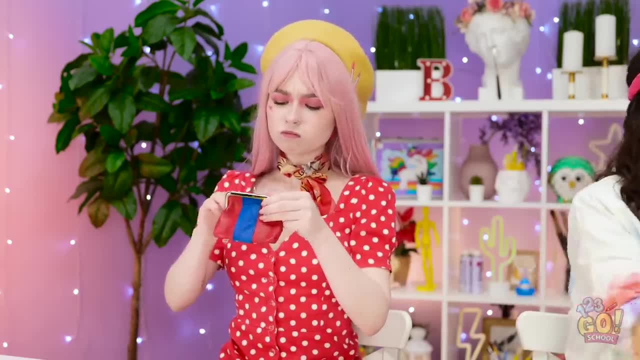 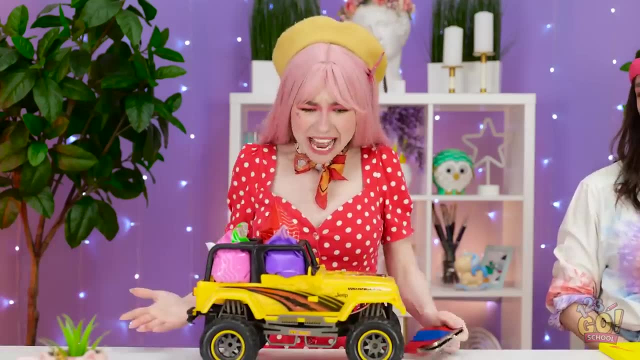 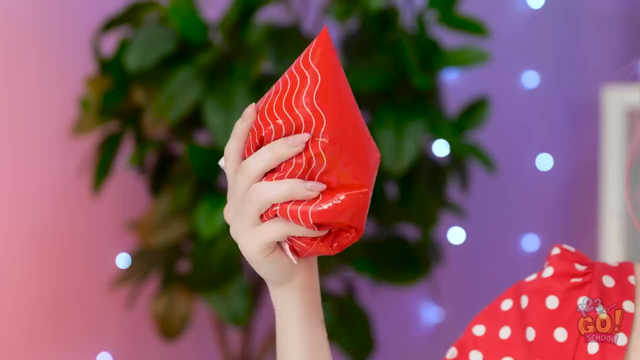 Wow, What am I supposed to do with this? Oh, I'll just buy what I need. Huh, What is this? It isn't paint supplies, that's for sure. What's in this thing? anyway, Wait a minute, I got it. 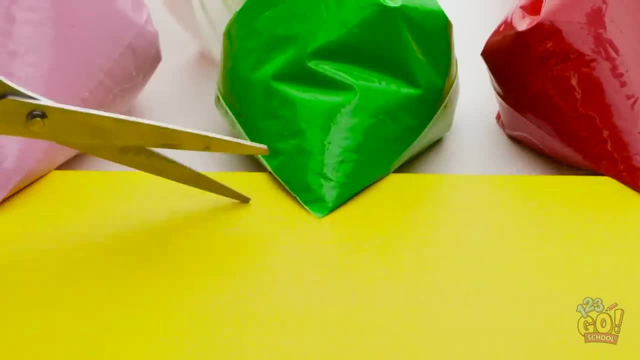 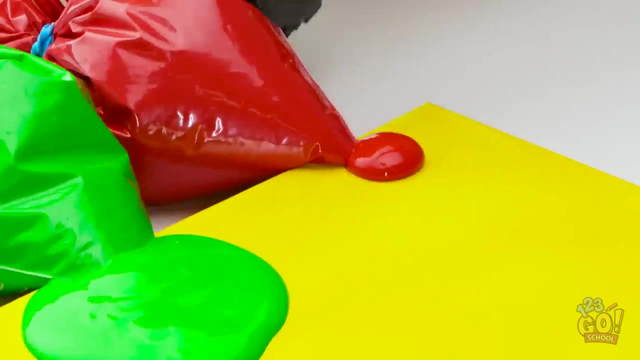 Just cut the tips off the bags. Okay, Okay, Just cut the tips off the bags. Okay, Just cut the tips off the bags. It creates a little spout thing. One more. Let the paint spillage begin. Oh yeah, Just look at all that stuff. 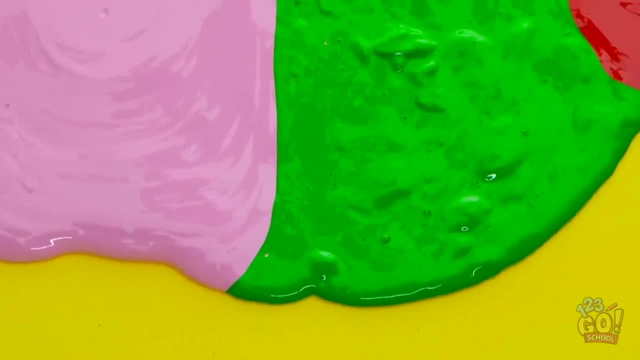 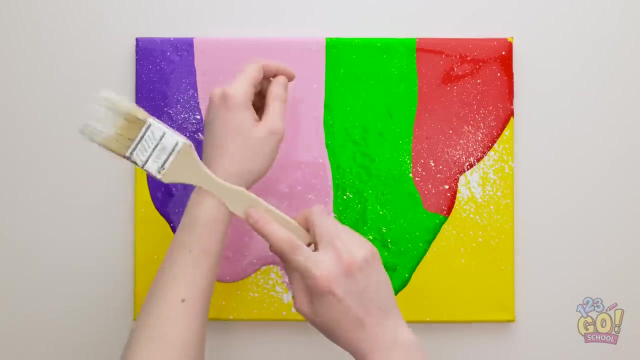 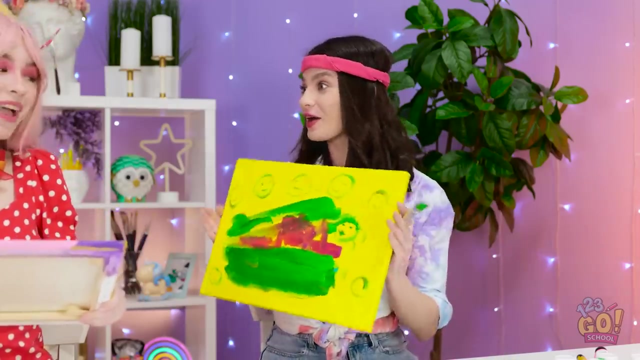 And now let gravity get to work. It's pretty fun to watch, isn't it? A little white will add a fun effect. Splish, splash. This is super cool. Just look at it. All done You like Super weird, right? 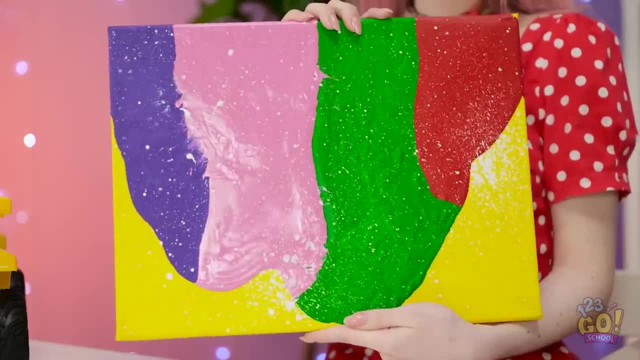 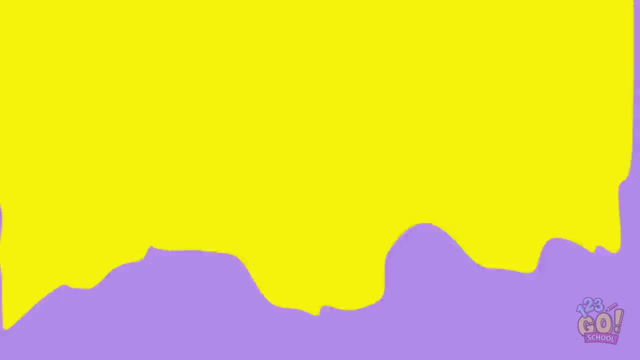 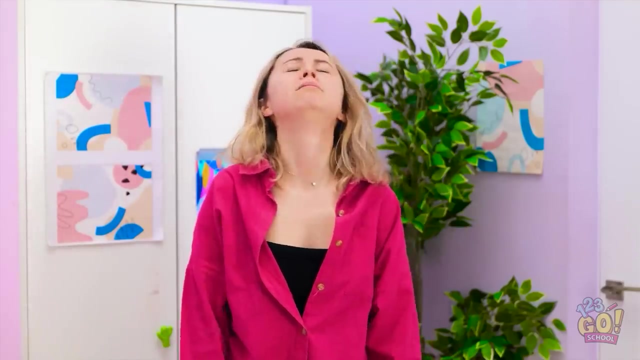 For sure, But look at this: How'd you get all that texture? I won again. You can't leave me, Mom. I'll only be gone an hour. sweetie, Now get up off the floor. Oh, I'll see you soon, okay. 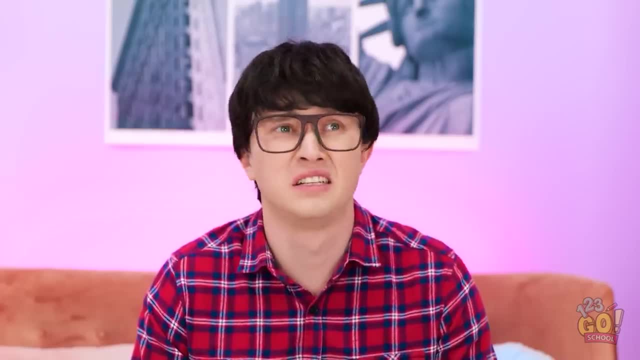 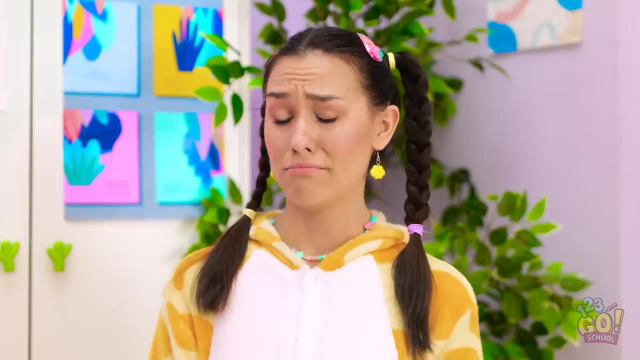 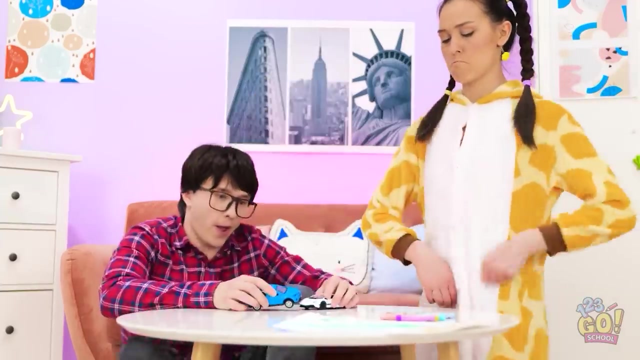 Play with your sister? Do I have to? Oh, look at that face. Don't worry, we can play. Let's race the cars. Yeah Well, I guess I can play that. I want the white one Get on the floor, okay. 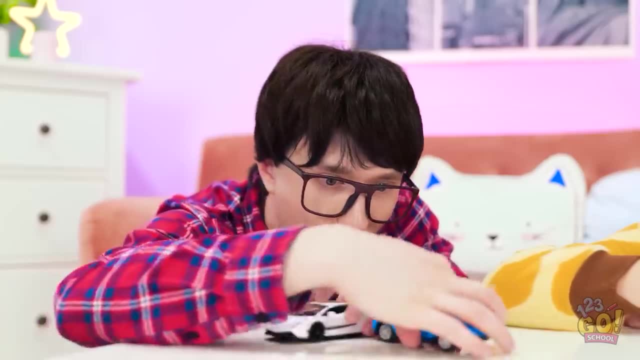 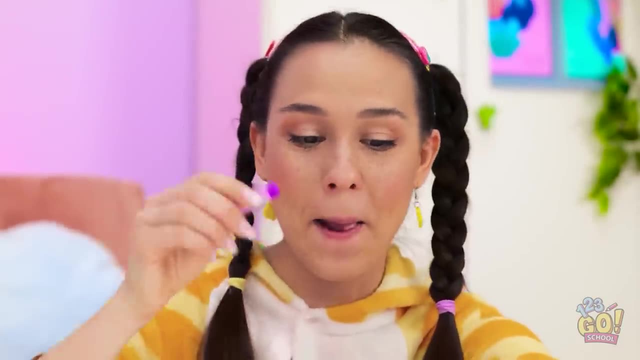 I wonder how long she'll be gone, As exciting as this is…. Why do boys love cars so much? Hey, I know how to make this more fun. I can just jump on the car and play. I can just draw on the table. 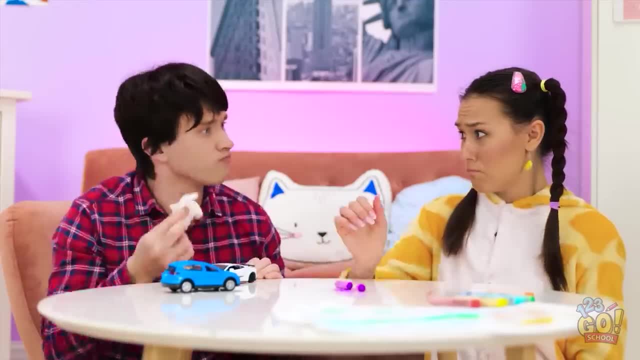 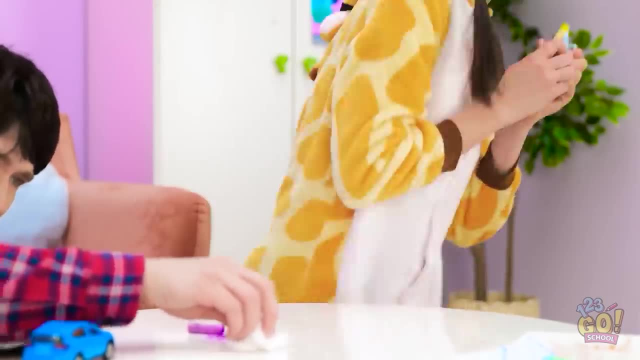 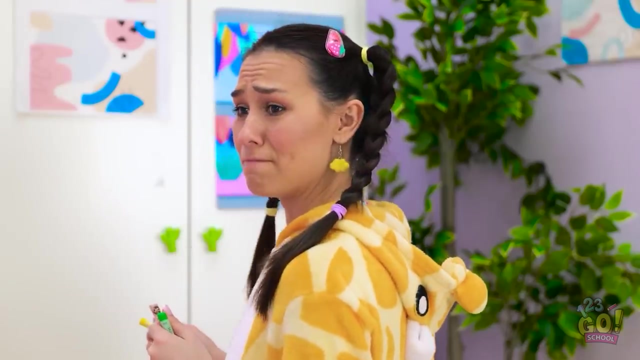 Are you insane? Very bad. Good thing I've got all these Aw man, I think I got it all. What can we do now? Everyone likes soccer. right, Come on, it'll be fun. Hey, watch this. 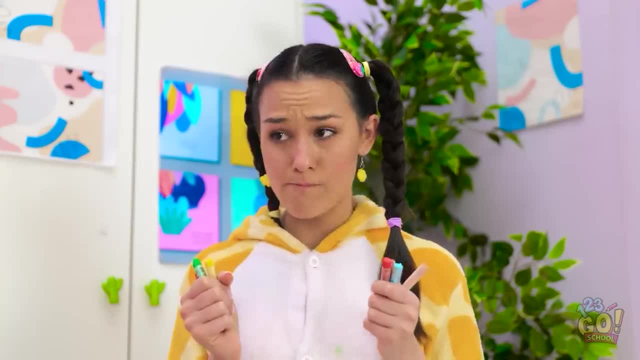 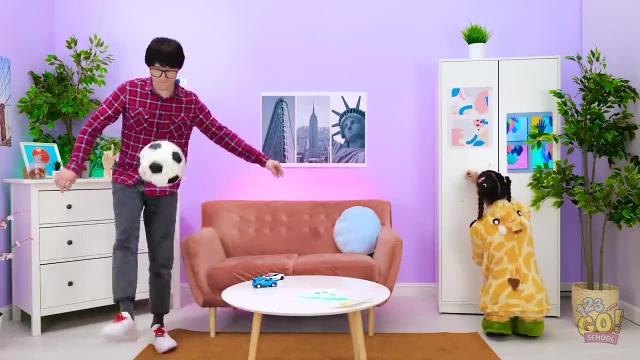 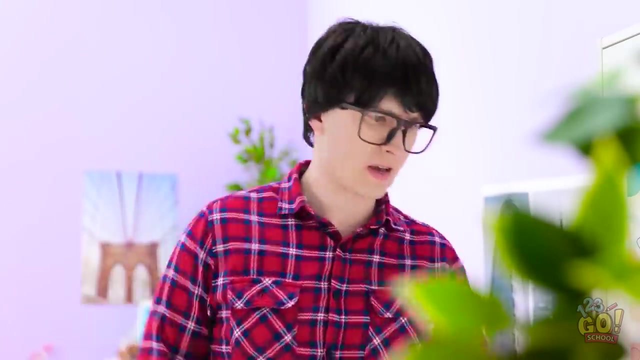 Catch. I missed, But it is fun, I guess. Hey check out this trick. Cool right? No, Gabby, What You can't draw on all the furniture, I told you, Uh sorry, But I know something I can draw on. 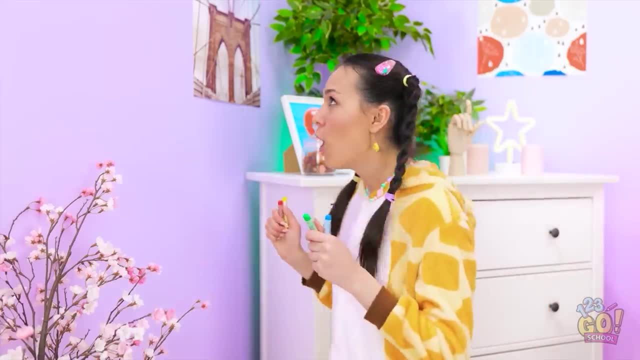 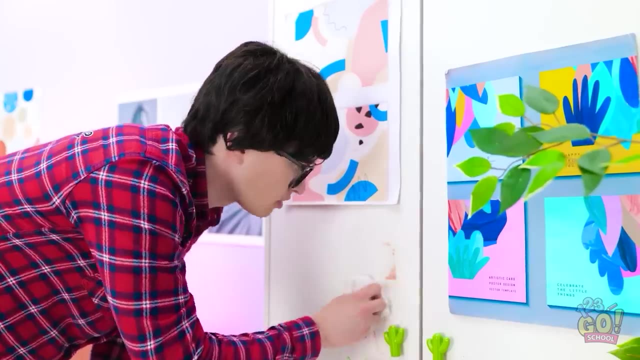 Oh, I've got all this wall space. It's gonna be my big house. I'm so excited. Let's go. I've got my big masterpiece Here I go. My arm is so tired. Gabby, where are you? 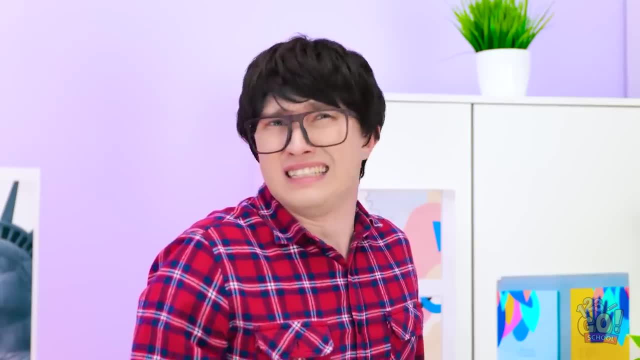 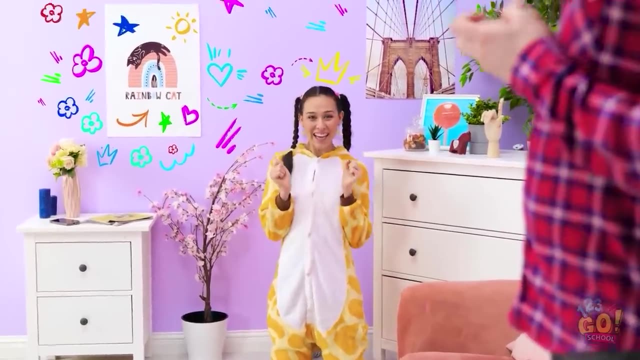 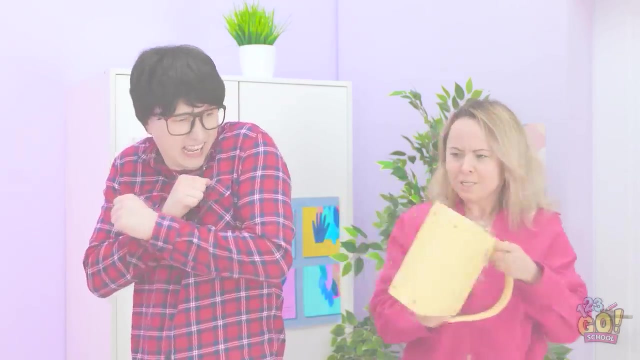 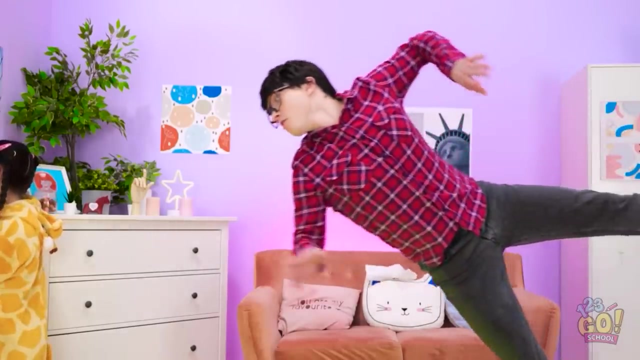 No, Oh gosh, I'm back. kids, What the You're home. Look what I made just for you. You're never watching her again, Ever, Ever. Hold up. I'm taking control here. Put the crayon down. 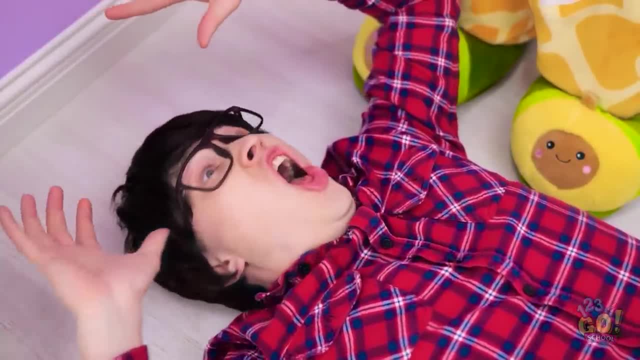 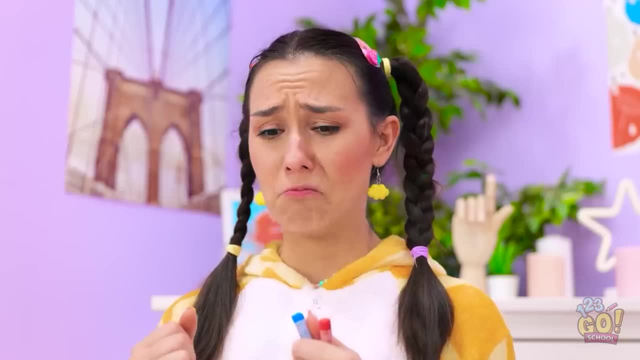 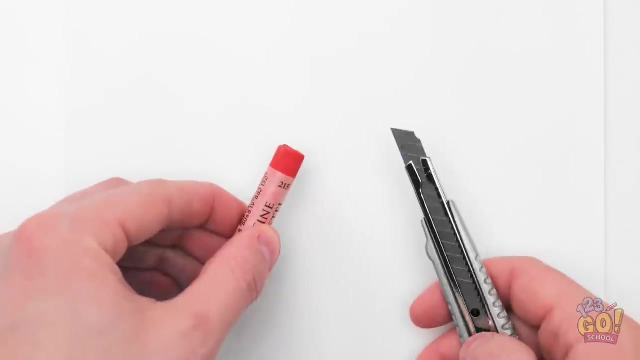 Gabby, don't do it. Put it down What. I can't take this stress anymore. Gah, That was my favorite crayon. Wait, I'm sorry, Don't cry. Wanna have some fun with crayons. Simply use a blade to shave them down. 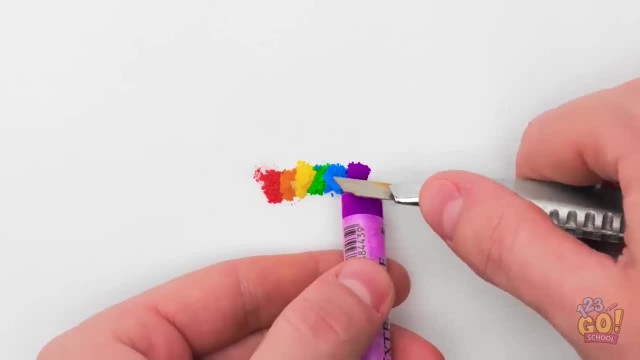 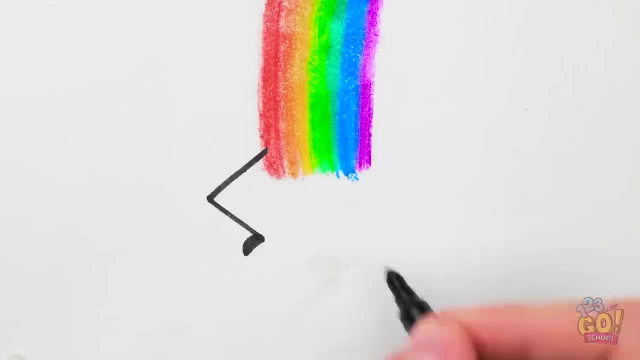 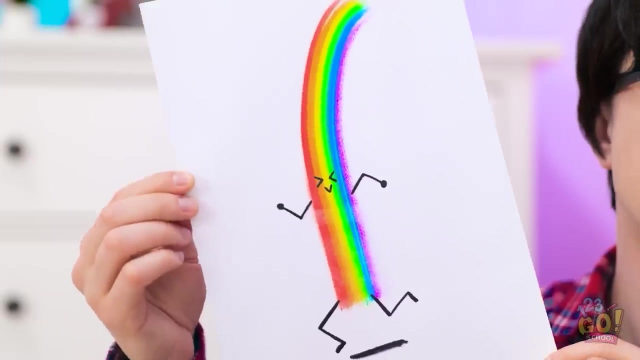 And use a bunch of colors, Then press and spread. You can even draw on it. I call this Mr Rainbow. Don't forget the legs There, Isn't he cool? I love it. Can I try Kids? I'm home. 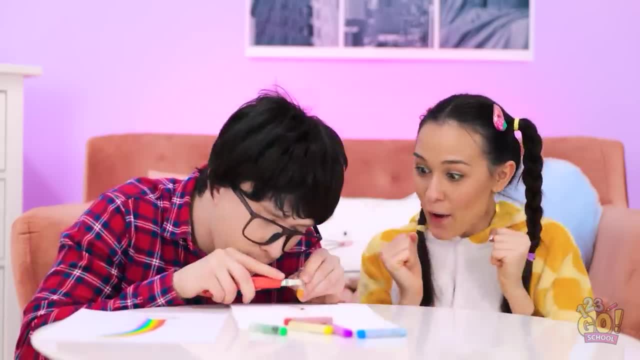 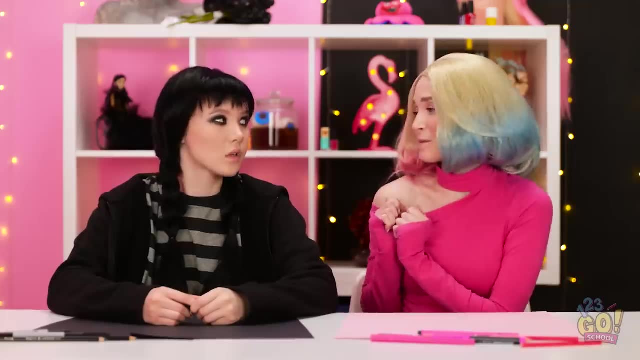 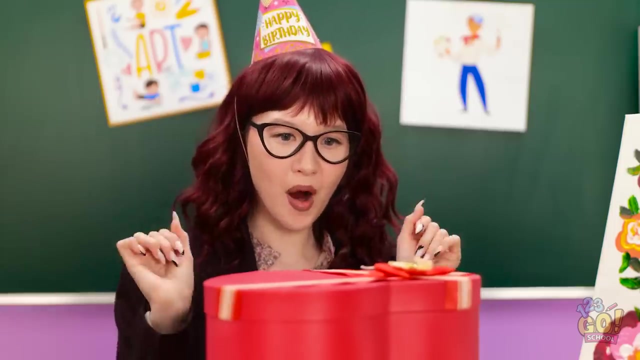 You have fun without me Again. Oh, I love seeing them play together. I got this new dress. It will look great on you. Here comes the teacher: Hi class. Happy birthday to me. Oh, what is this? I can't wait to open it. 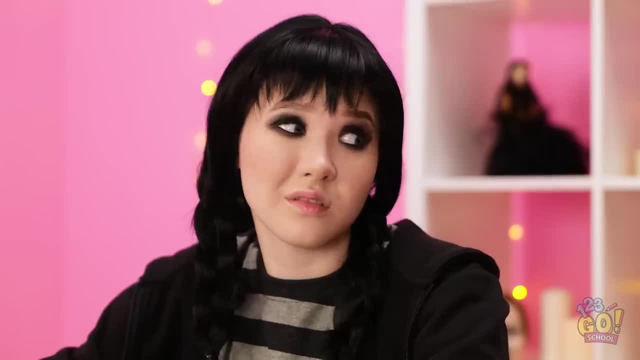 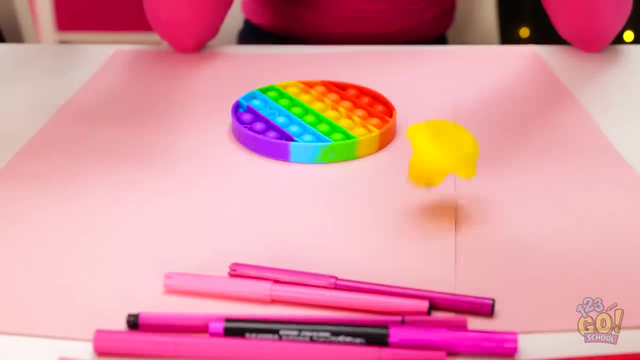 Wait, it's her birthday. I don't have any gifts, So Who cares? I need to give her something. I know I must have something in my bag. Hmm, I can't give her a rubber duck. No, none of this will do. 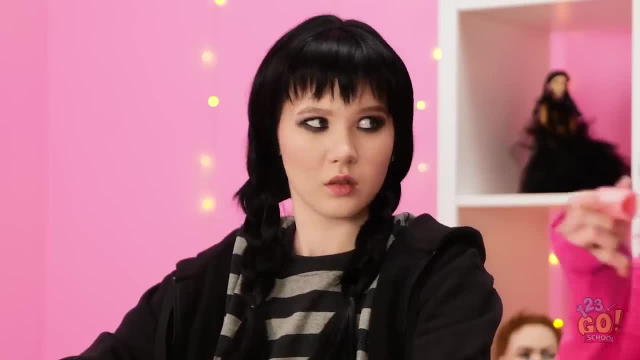 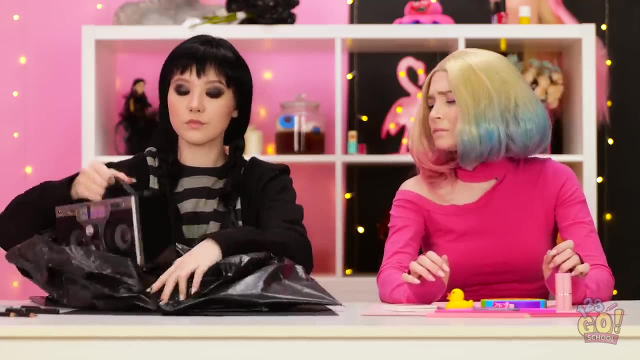 I'm out of ideas. You're giving up that easily. Okay, let me have a look. Maybe I have something we can give her. You carry around a trash bag, Ah, okay, I get it. Do you think she'd like bugs? 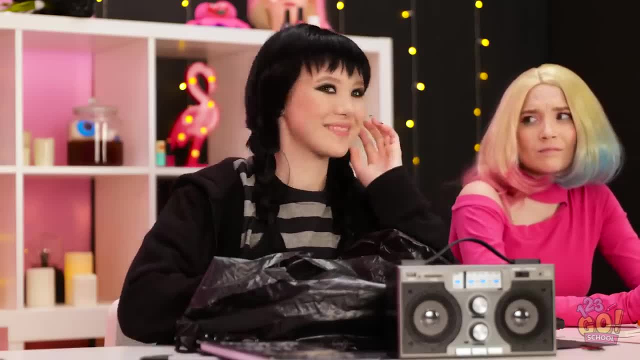 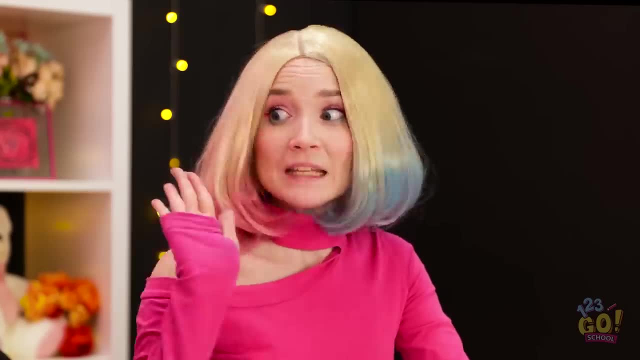 Uh, no, ugh. Hmm, I can't let Ashley see this. Love you, Teddy. Now where was I? Nope, I've got nothing. It's okay, I'll make a call. Hello, It's not a big deal. 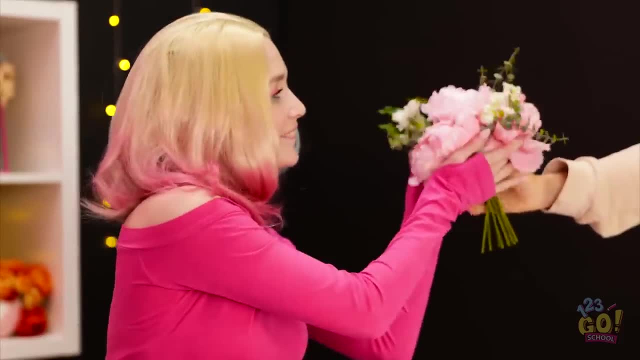 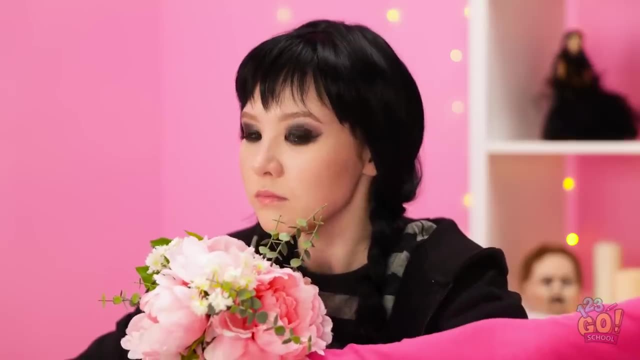 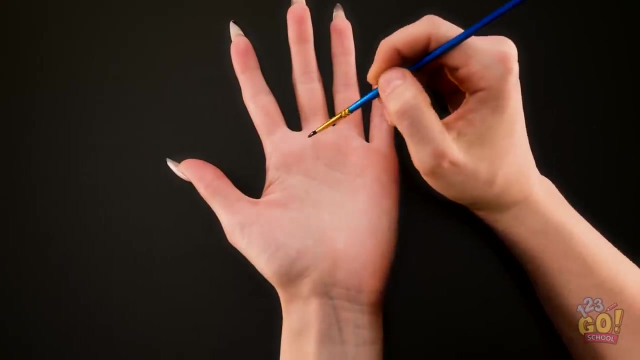 Thanks for your help. Whoa, That was quick. Hmm, they smell amazing Flowers, But they're beautiful. Go on smell them. I hate flowers. I mean, I'm allergic. Hmm, that gives me an idea. I'll paint on the palm of my hand. 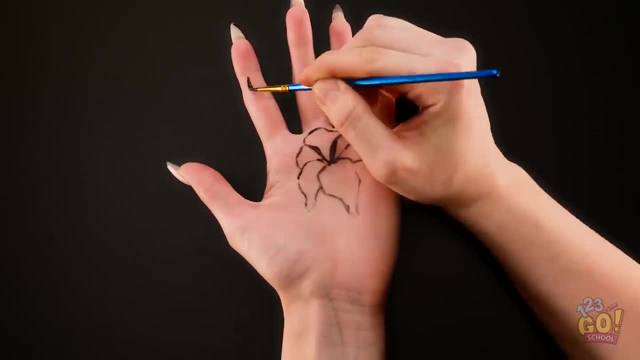 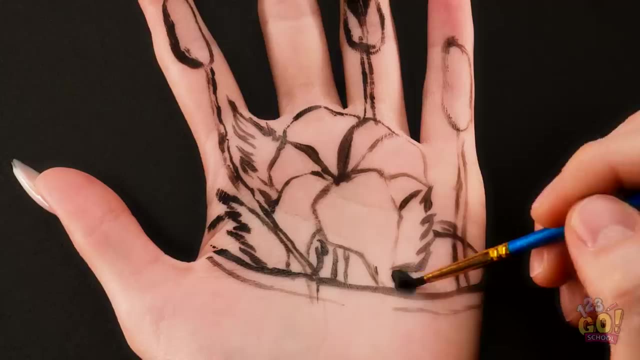 I want to create a flower. I'll draw the leaves and petals on my fingers. It's important I do this against a black background. It really helps create something special. Once that's done, I can start filling it in. I want to cover a lot of it with black paint. 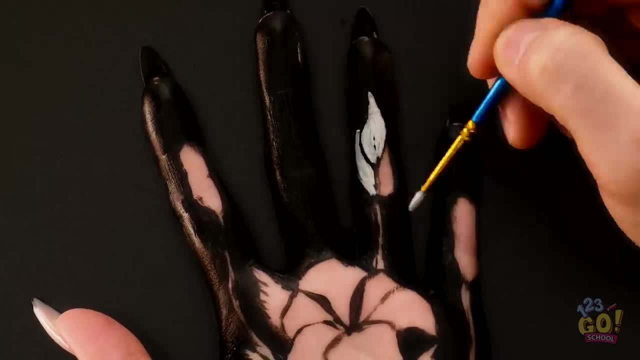 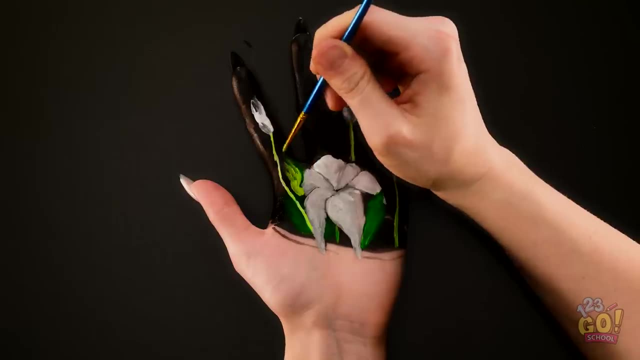 Then I can add color. I'll use silvery white for the petals- It just makes them stand out. Then I'll use a vibrant green. for the leaves I'll use a lighter shade to create contrast. Then it's a case of adding the finer aspect. 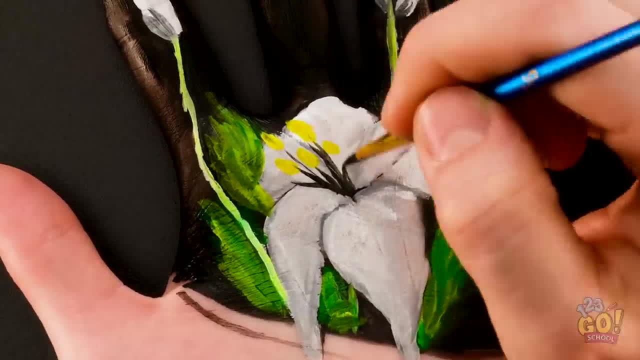 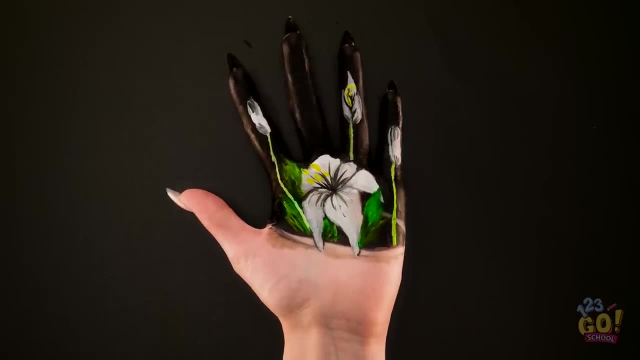 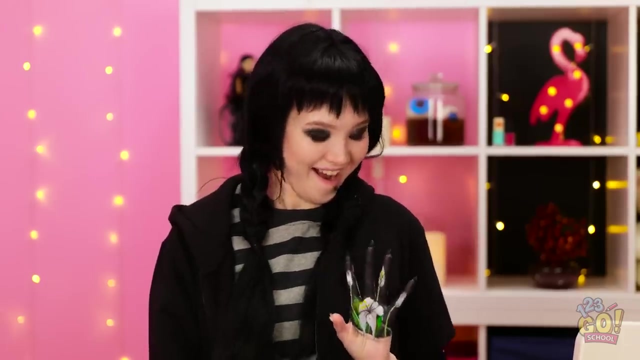 I'll go around the petals giving them details And I'll add an outline. I think that should do it. I'm pretty happy with that. That's my kind of flower. Hey, Ashley, What do you think? You like it. 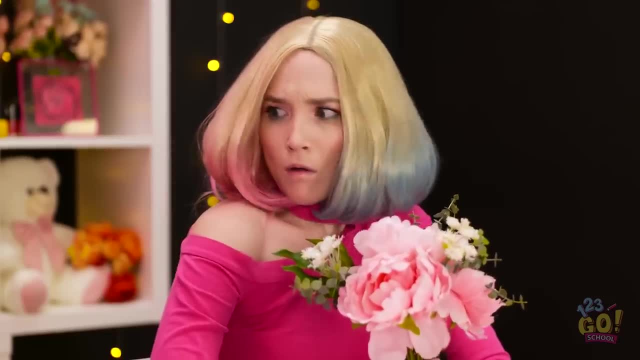 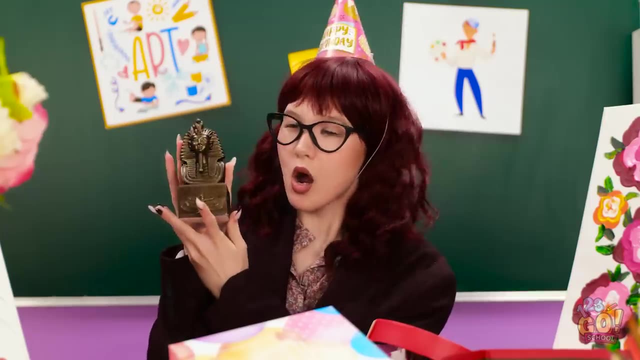 You like flowers, right? Huh, Did you do that? Yeah, I thought it might come in handy. Get it, Let's give them to the teacher. Hey teacher, Oh, Yes, what is it? I got something for you. 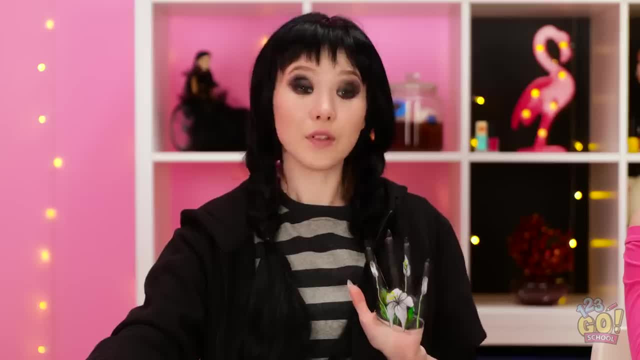 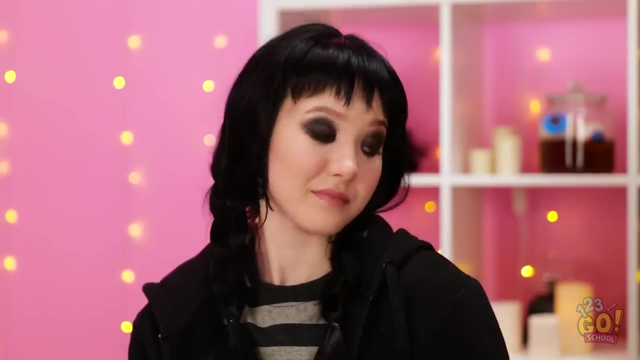 Really. For me, That's too kind. I got you something too. Whoa, It's beautiful. I've never seen anything like it. Hold on, I need to take a picture. I love it. Oh, I think she likes it. 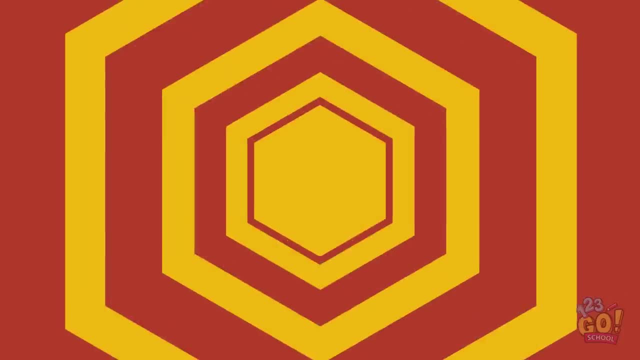 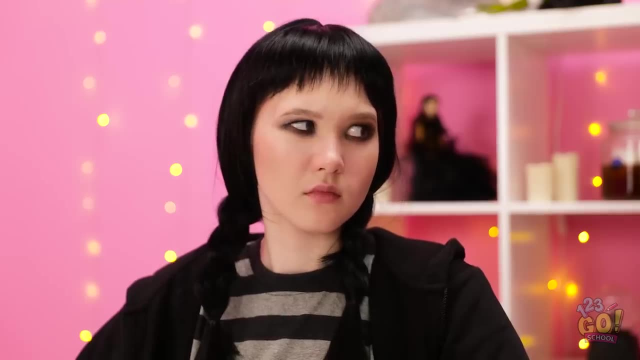 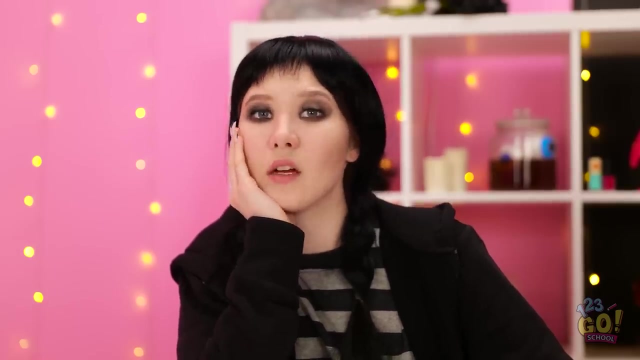 This is the best birthday ever. It's important to stay hydrated. I'm thinking of getting a new style. Any ideas? Why are you asking me: Just dye it black. You know I was thinking you should go blonde. Yeah, that's not gonna happen. 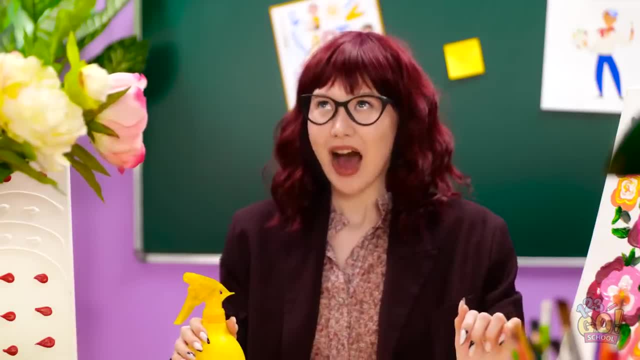 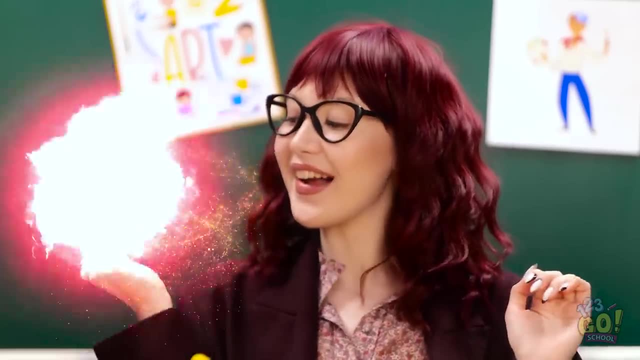 Hey, can we have something to do? Huh, Oh right, Let me think. Oh, I've got it. How about a little magic? Ladybugs are always cute. On you go. Whoa, Look at that, This is so cool. 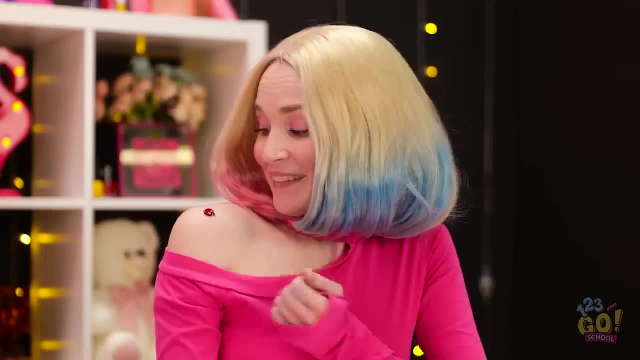 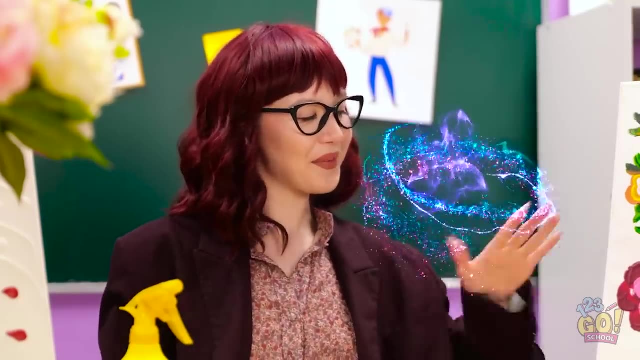 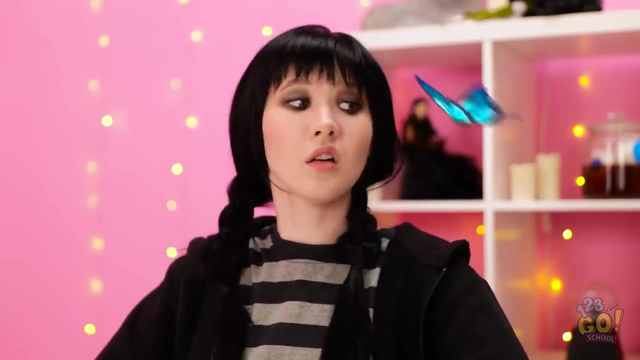 I feel like a cartoon princess. Whoa, Thanks. Now what about you, Mindy? Hmm, I've got just the thing I think you're gonna like it. Wait, Not so fast, Stay back, I mean it. 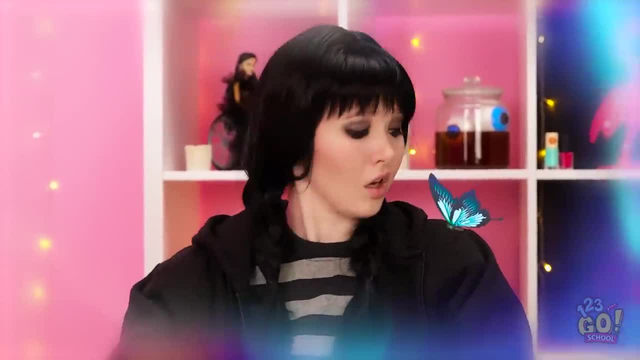 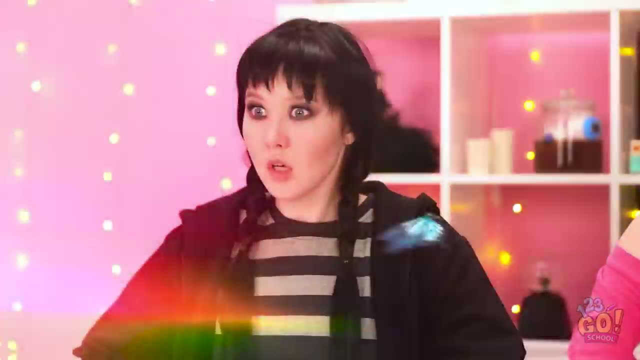 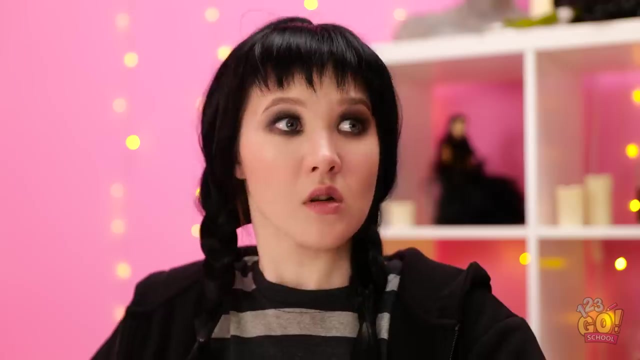 Make yourself comfortable. What, What's happening? Okay, that's never happened before. Whoops, I'm colorful. No, I don't like that. Get away from me. Ooh, I love butterflies. They make me so happy. 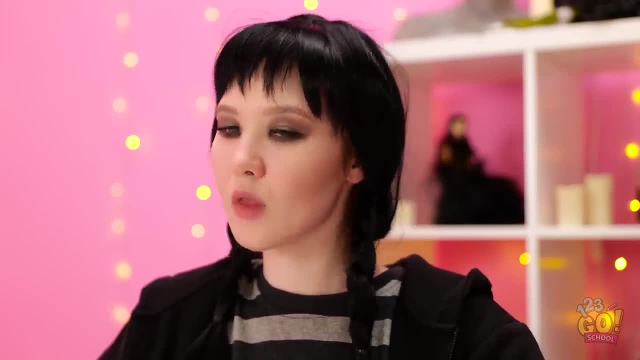 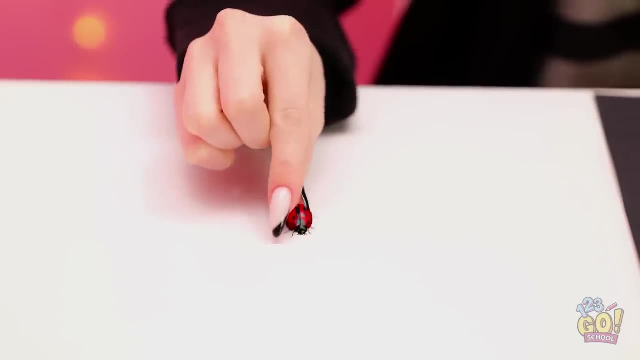 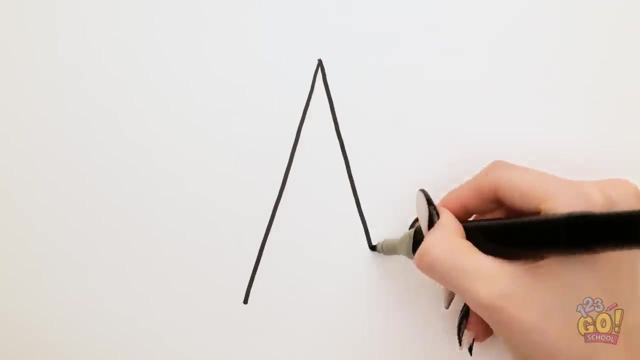 Phew, That was close. Hmm, I still don't have anything. Wait a second, Maybe I can use the ladybug. Don't be scared, You can go right there. That's it. Strike a pose. You've inspired me. 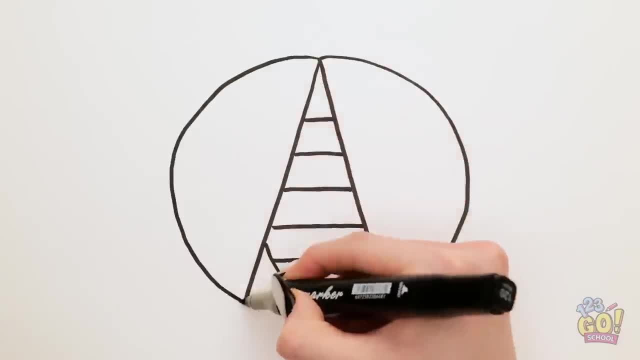 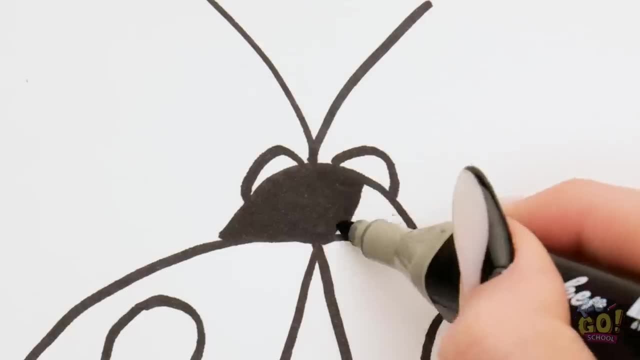 I'll start by drawing a triangle, Then I'll add some lines. Now I'll draw a circle around it, Then the head and antennae. Every ladybug needs dots. I'll color the dots with black ink. That's perfect. Then it's time for some red. 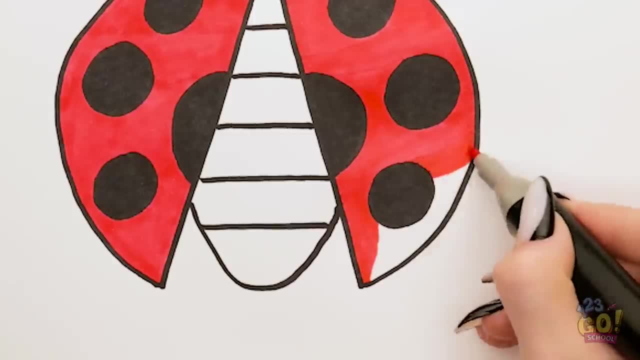 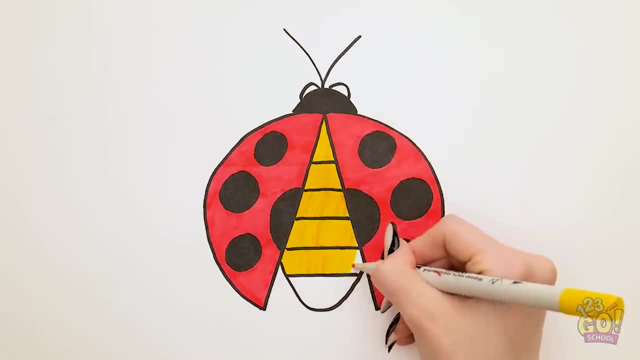 I'll just go around the dot. I don't want to ruin it now. This red is so bright I'll color the inside yellow. That's it, My own ladybug. It looks great. What do you think? I think I nailed it. 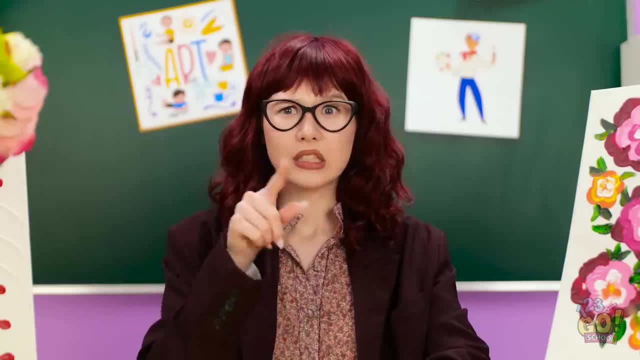 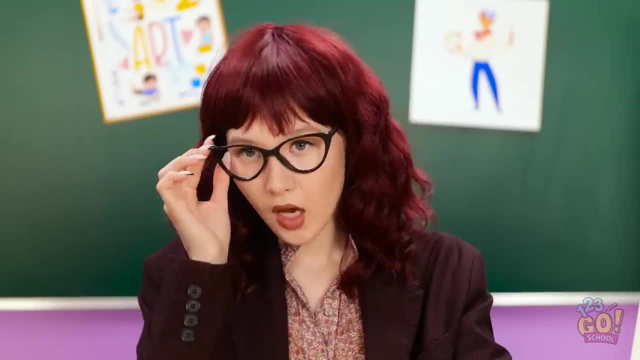 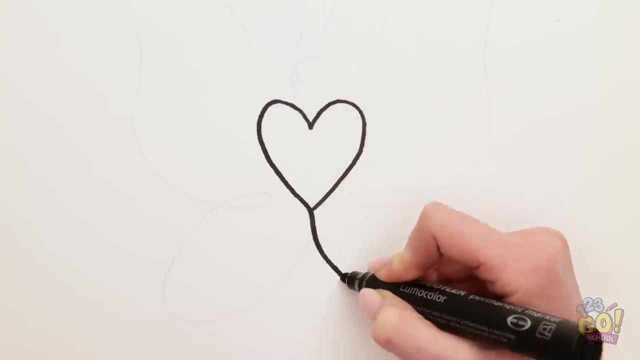 Wow, Wow, It's like looking in a mirror. You're so talented, Mindy, I'm impressed. I think we're gonna be great friends. Uh, Ashley, Hey, Huh, What is it? Oh, Give me a minute. 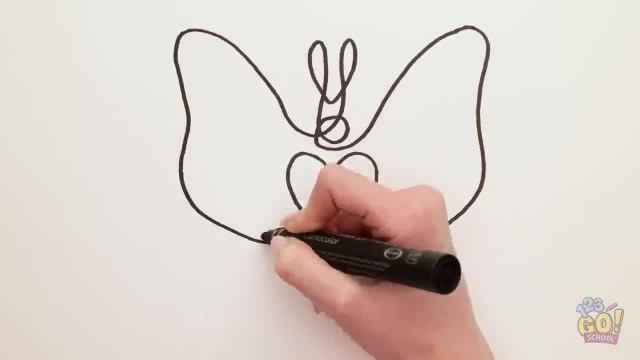 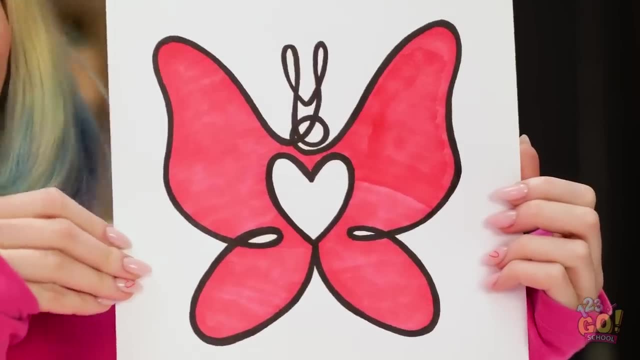 I'll draw a love heart. It's coming out of it. This is gonna be the wings- A splash of red and it's done. There you go. It's pretty, isn't it? Oh wow, Nice work Ashley. 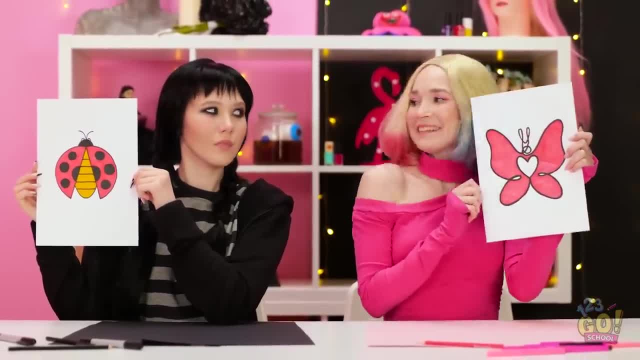 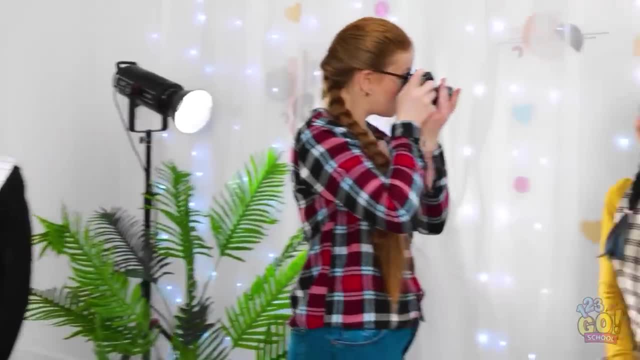 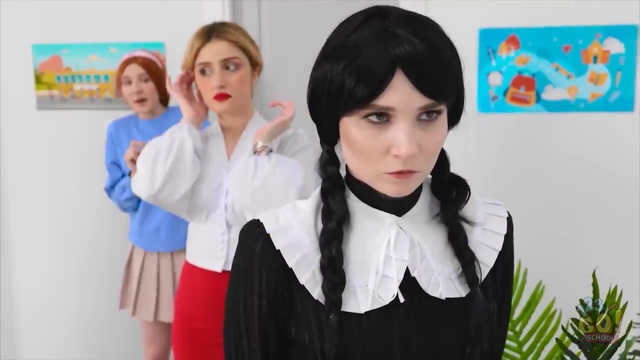 I'm so lucky to have you both in my class. I love your ladybug. Ooh, I am looking good. Ugh, Oh yeah, That's it. We're all done here, Right? Who's next? That would be me. 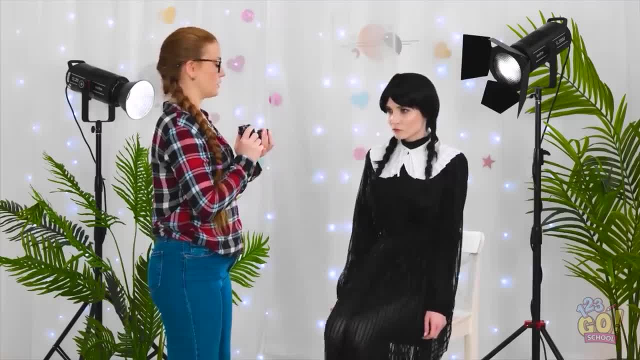 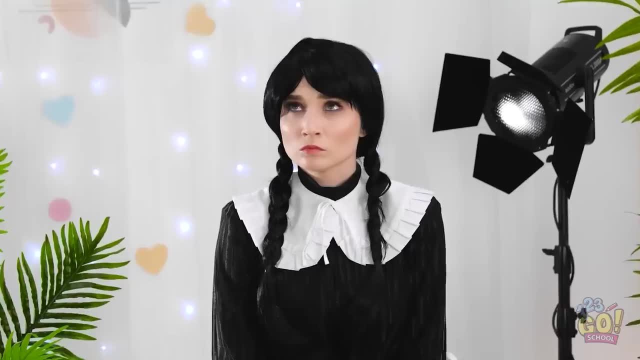 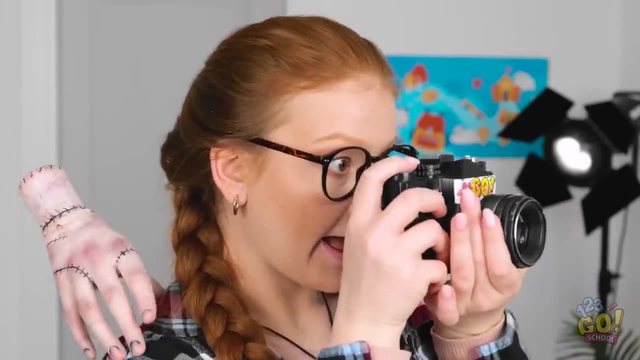 Let's get this over with. Whoa, I love your style. I can work with this. I love the monochrome look. How about a smile? How about no? Okay, You like the moody look, I get it. What is it? 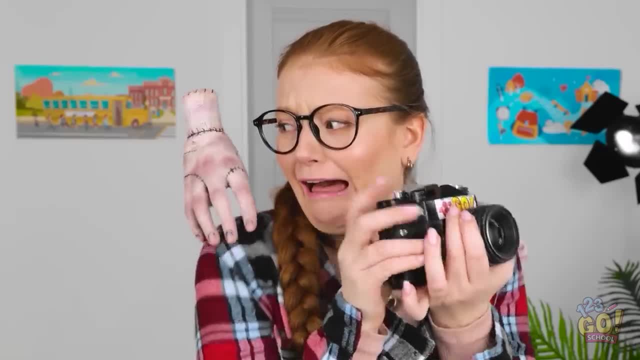 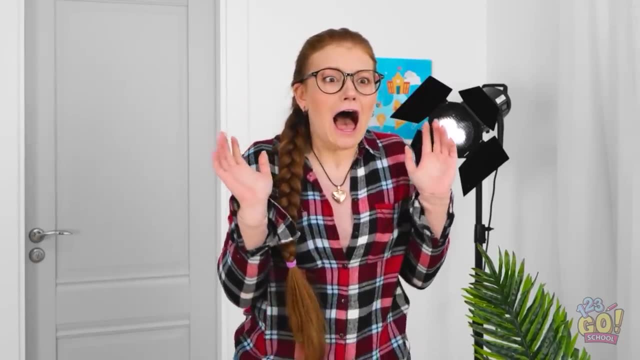 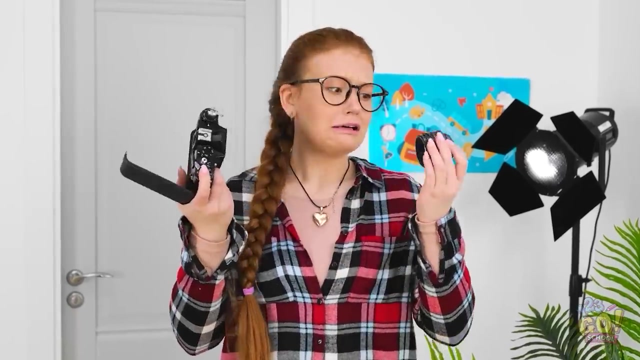 Is that a hand? It's with me. This is so weird. Get off me My camera. Oops, I can't use this, It's ruined. How am I supposed to take photos now? Hang on, Maybe I can use this. 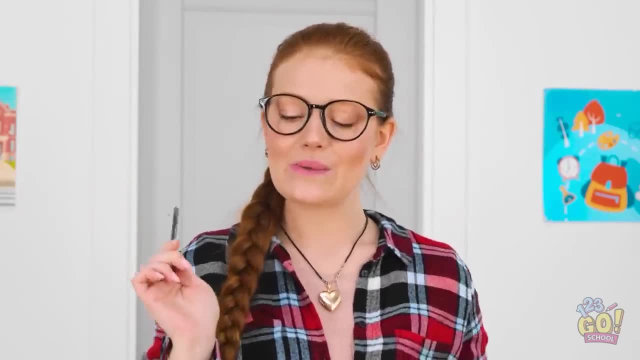 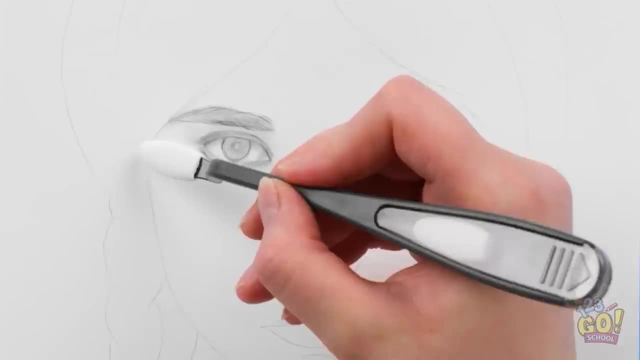 I think it might work. It's worth a shot. Just stay there. I'll just sketch out your face, Then I'll go over it with heavier lines. I'll take my time. This will give me shading and texture. It helps make the drawing look more realistic. 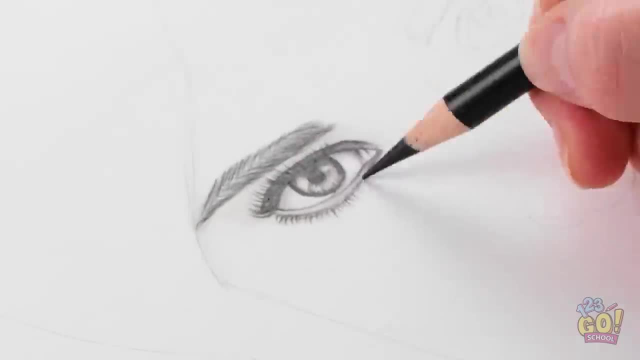 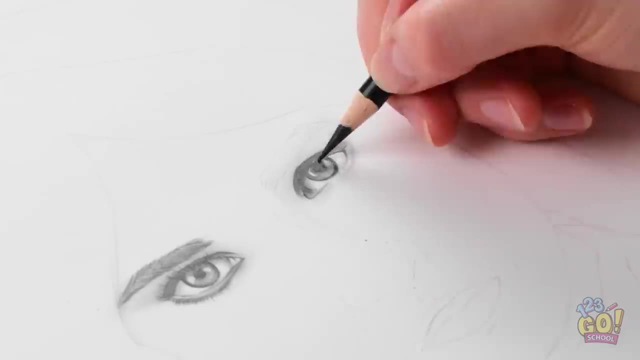 Wow, Those eyelashes look great. I wish I could do my mascara like this. Now for the other eye. I really want to capture your essence. The eyes tell a story. Smudging the drawing gives me shadowing. I can use this special tool for that. 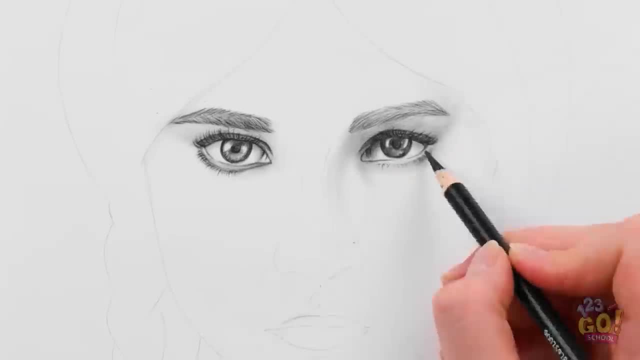 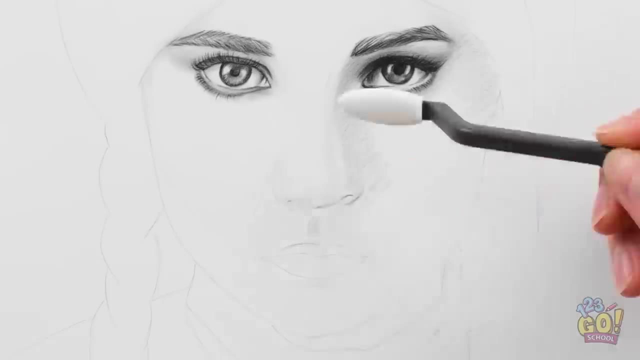 And it stops my hands getting dirty. Using a white pencil gives me contrast. It helps give the impression of light and darkness. This is going well. Now for a little shadowing around the eyes. This will accentuate the natural curves on your face. 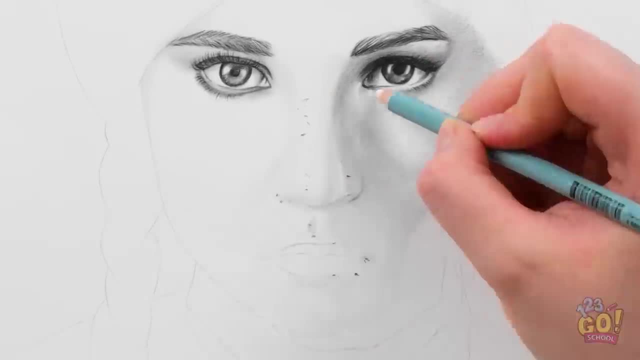 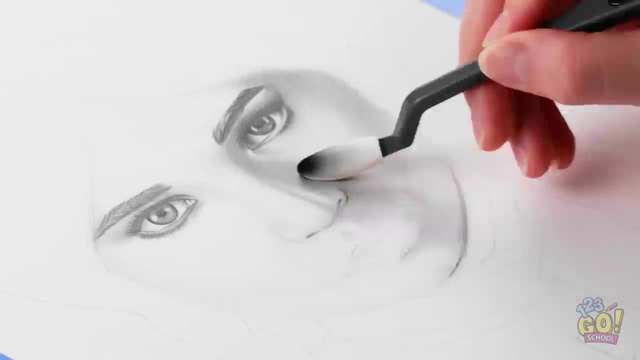 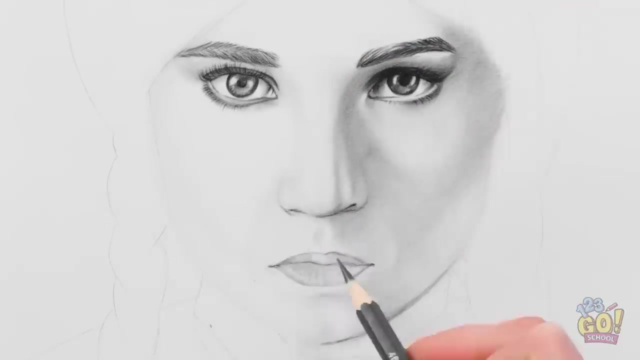 Those cheekbones are poppin' Wow. Now I'll add a little more detail around the eyes. You can't rush perfection. It's really coming together. Next I'll work on the lips. Mixing the light and dark pencils gives depth. It makes it stand out. 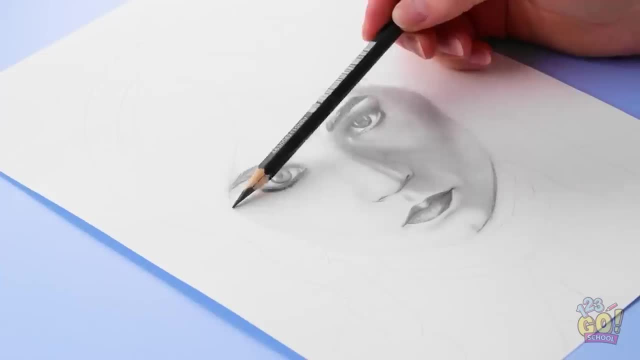 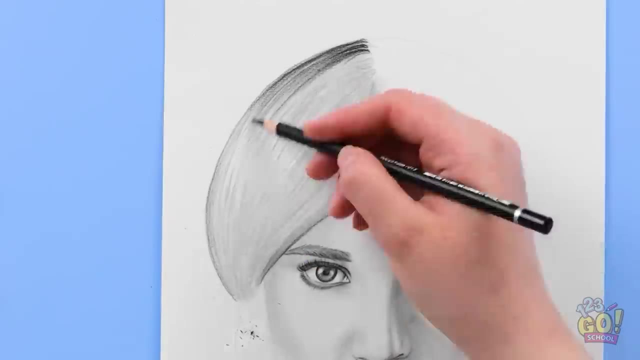 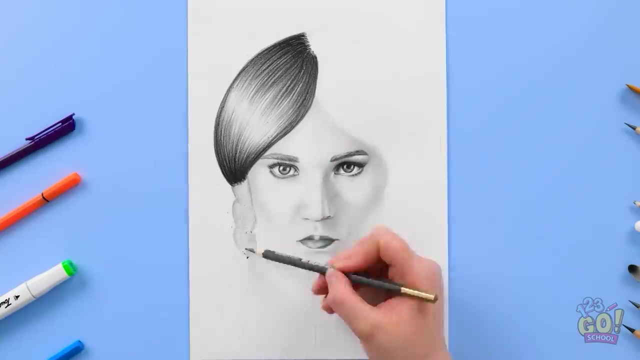 And the drawing comes to life. Now it's time for the hair. Using light and heavy lines helps give the impression of hair. I'll leave a gap in the middle. This will be the light reflecting. Then I can work on the braids. 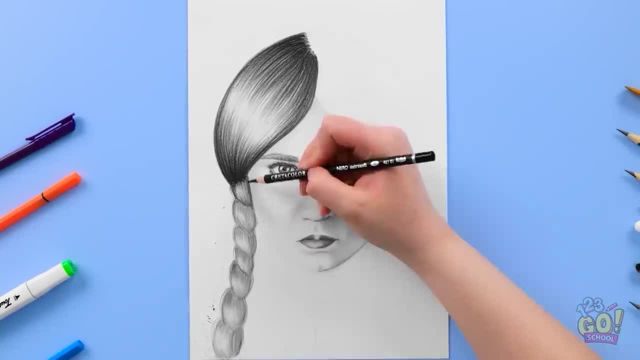 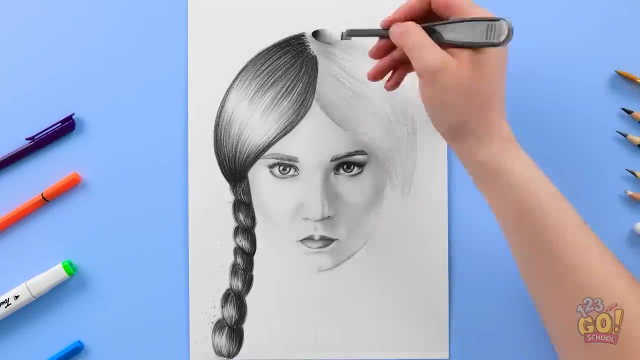 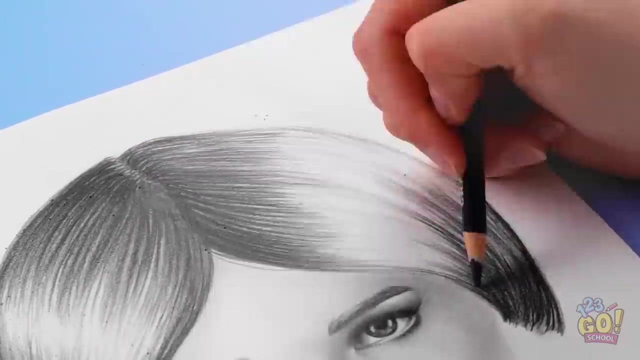 I'll keep going over the braids. It'll make them fuller. Then I'll do the opposite side. It's just the same process: Building up the layers and the texture. I want to keep the light reflection in the same spot. Now I can start to work on the body. 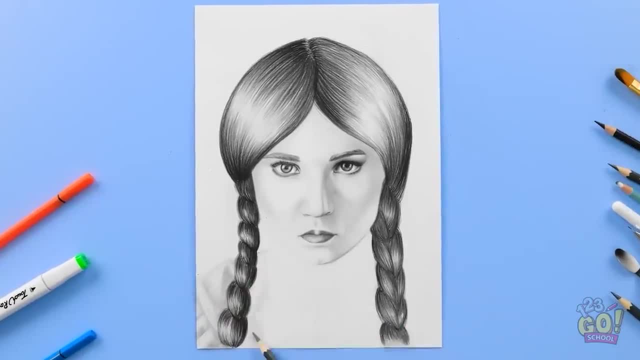 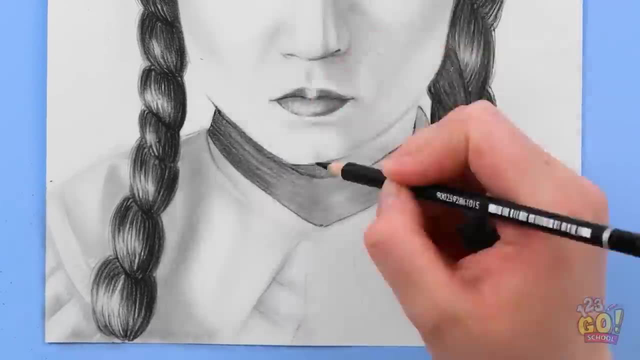 I'll go over it lightly And use the blending tool to create shading. I'm glad you're not wearing multicolored clothes. It makes my job so much easier. Once I've sketched it out, I'll go over it with black pencil. 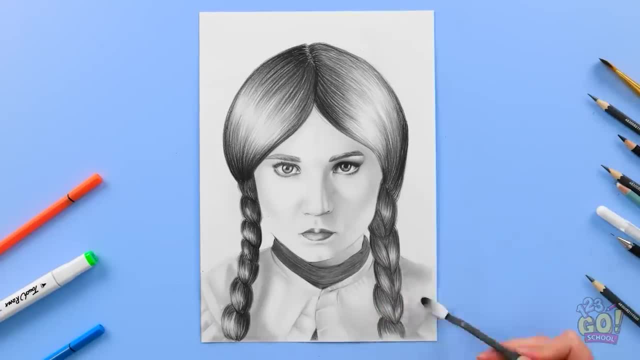 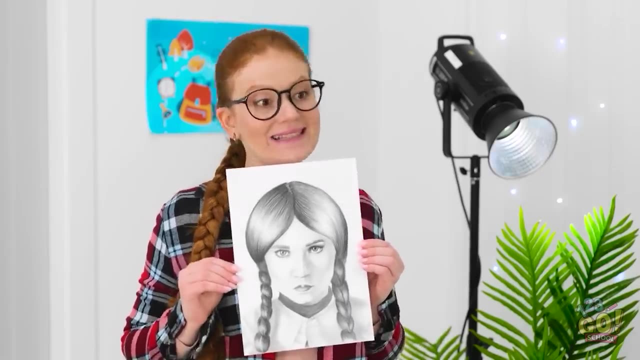 I'll apply more pressure. I think it's finished. It's better than any photograph I've taken. I've really nailed your creepy stare. Check it out. What do you think? I hope you like it. Is that me? I look so pretty. 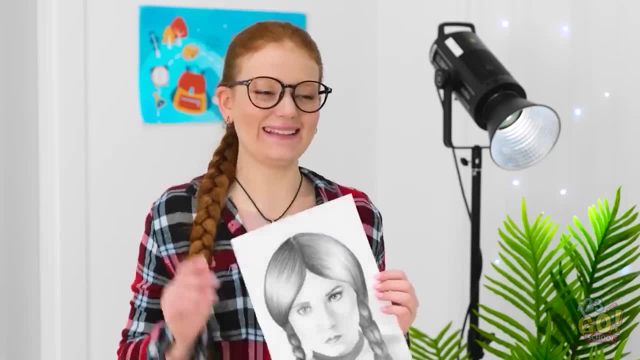 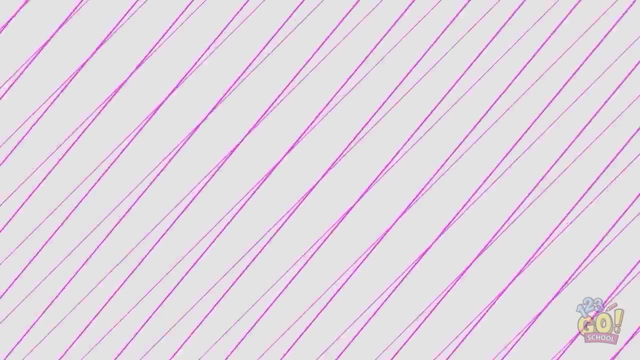 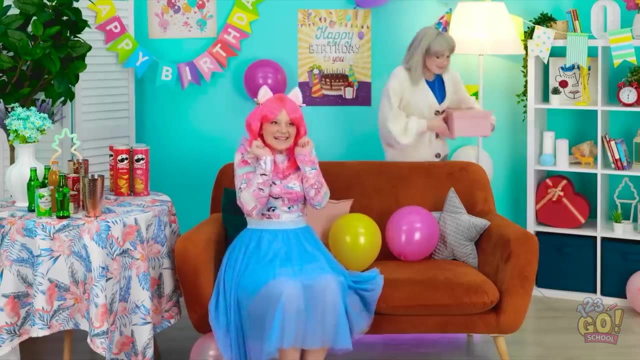 You're so talented I was getting worried for a moment. I thought you were going to set the hand on me. Here you go. Phew, Now get out of here. Can I look now, mom? Happy birthday, Yay, Thanks, mom. 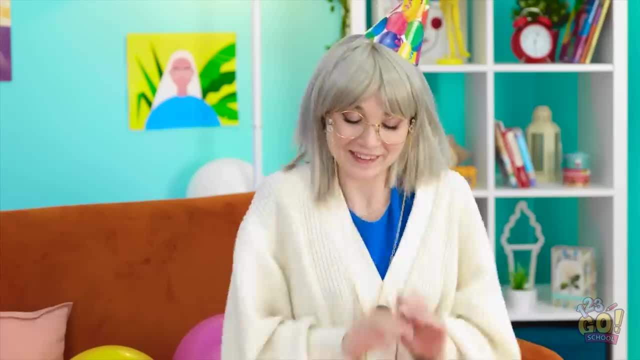 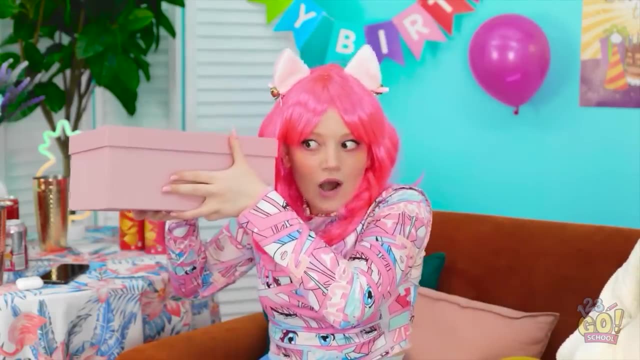 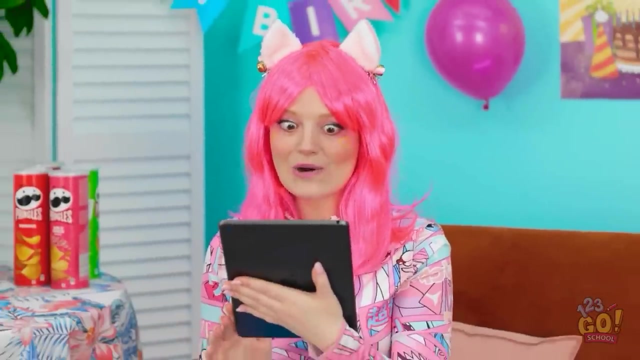 I've got something for you, Really For me. You deserve it, honey. Wow, I wonder what it is. Ooh, This is so exciting. I love surprises. Whoa, Is that an iPad? Wow, Thanks, mom. 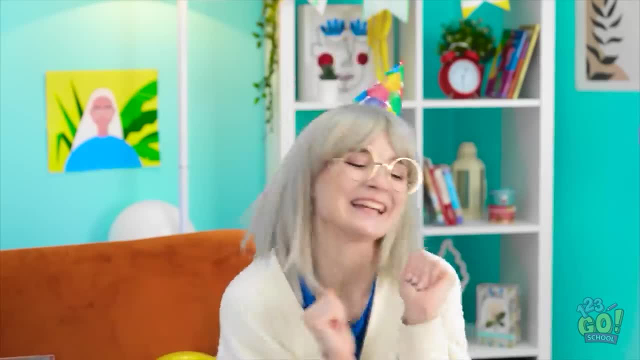 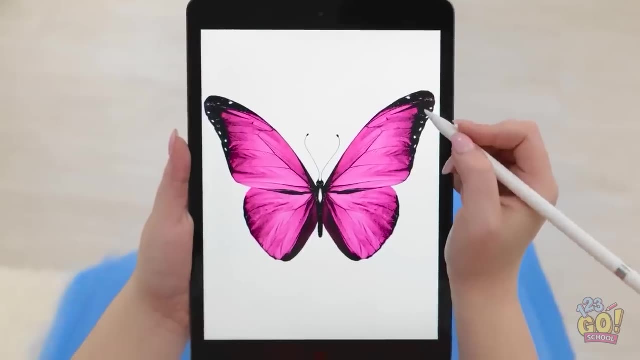 This is awesome. I'm so happy. I love you, honey. Hmm, I have an idea. I'm going to draw something. Ooh, This is good. It's a beautiful butterfly. Wow, That was so easy. Wait, What's happening. 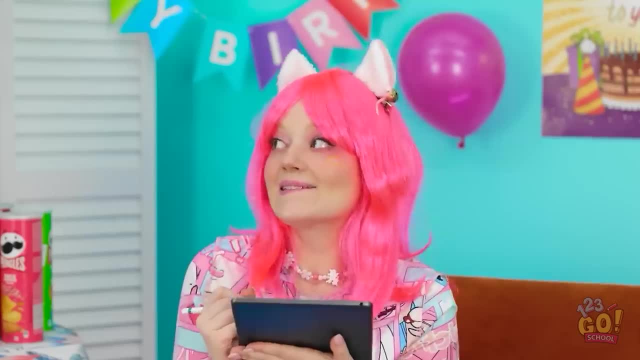 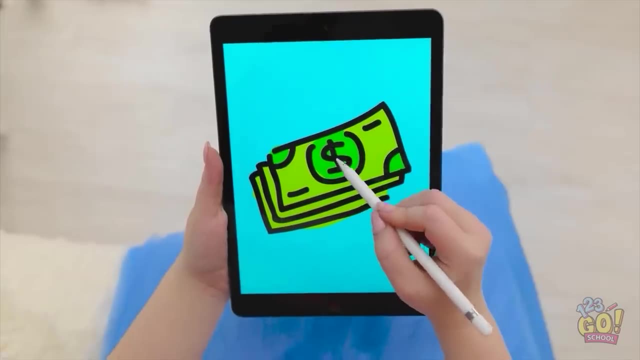 Wow, Look at that. It's so magical. What else should I draw? Hmm, I have an idea. Should I? Yeah, I'm going to do it. I'll draw a large pile of cash, And now I wait. Something's happening. 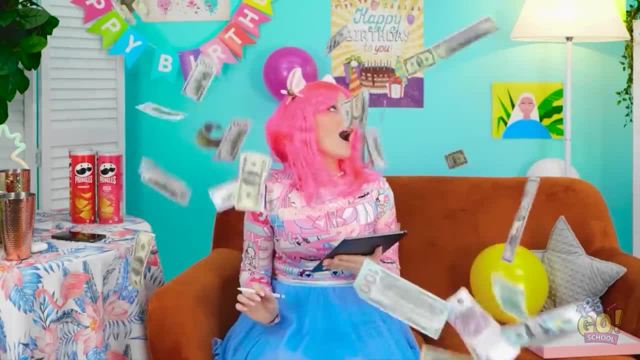 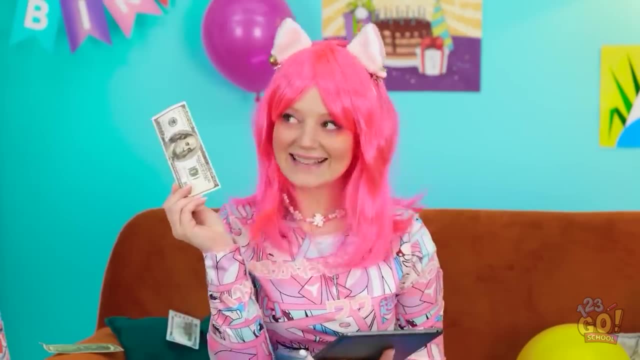 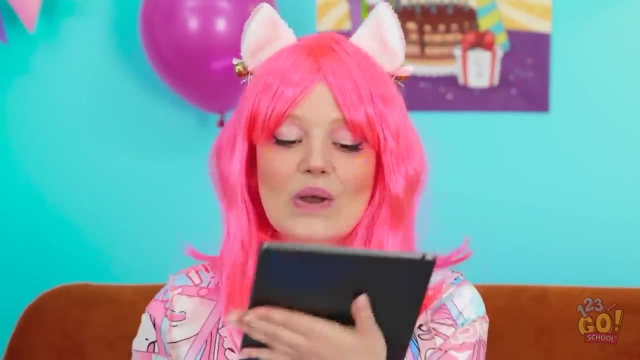 I think it's working. Whoa, Look at all this cash. Whoa, I'm rich. I've never seen so much money, And it's real. I'm going on a shopping spree later, But first I've got something else to draw. 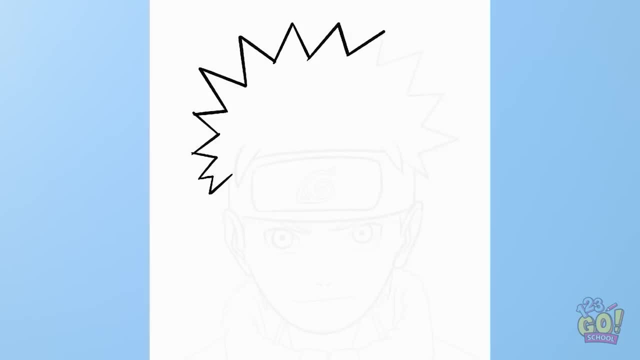 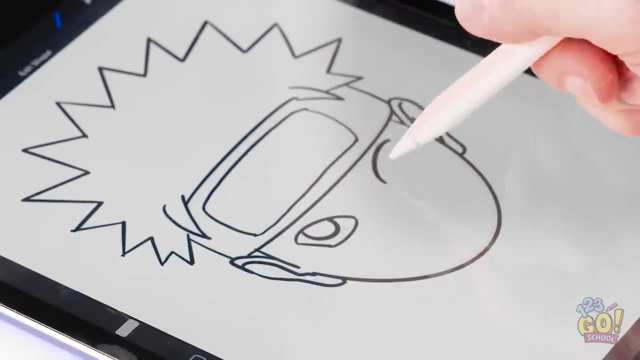 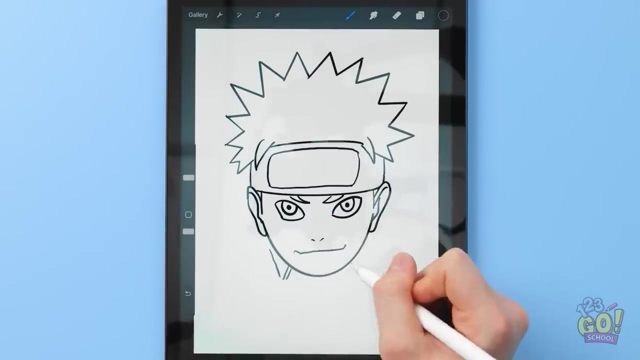 Here goes: I've sketched out a fame outline, Then I'll go over it. Now I'll draw the eyes- It's looking good already- And next I'll do the nose and the smile. I like this. And now for the body. 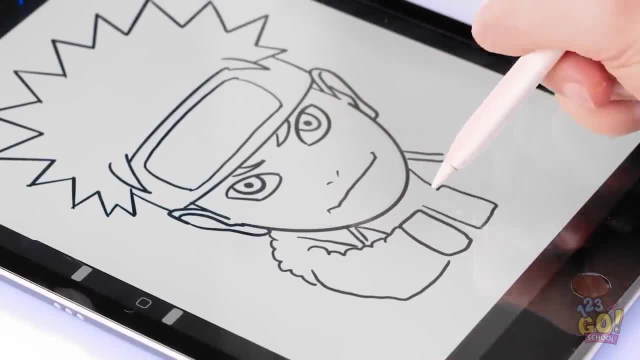 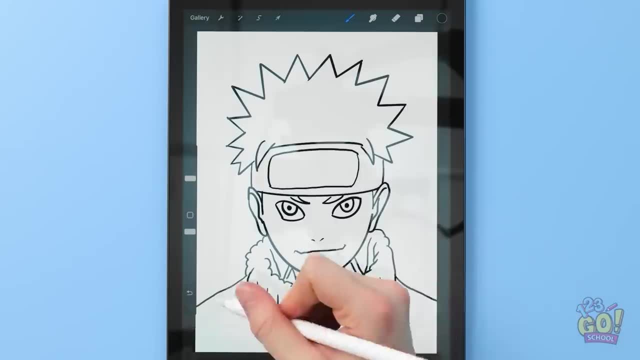 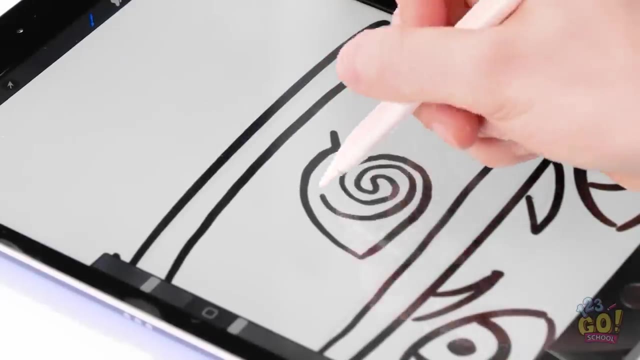 That's one cozy-looking jacket. I wouldn't mind one of them. That's the main part's done. I can start working on the finer details. I'll create the logo on the bandana. This can just be a spiral. It's time to add color. 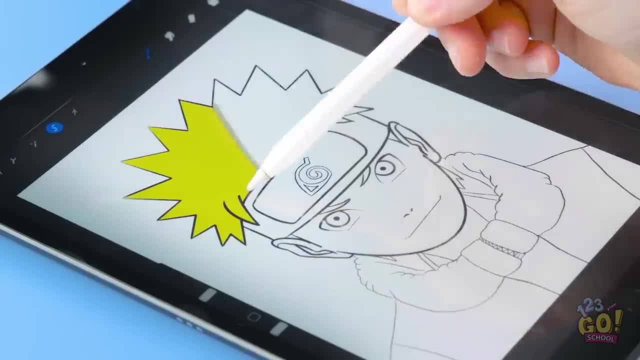 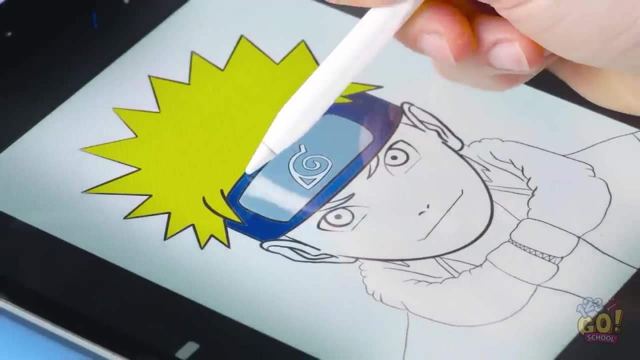 I'll use yellow for the hair. I think he suits being a blonde. I'll use blue for the bandana. I'll use different shades of blue, Then I'll add shadowing. I want to create contrast. I'll give a metallic look. 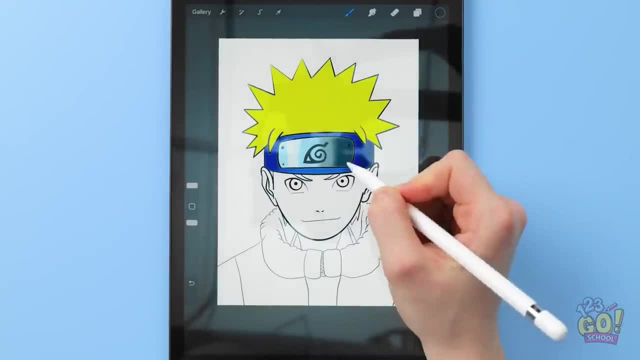 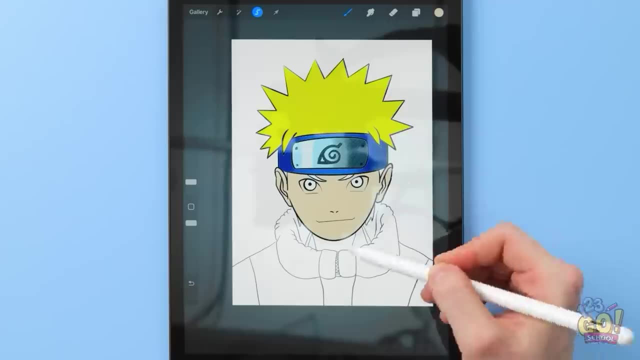 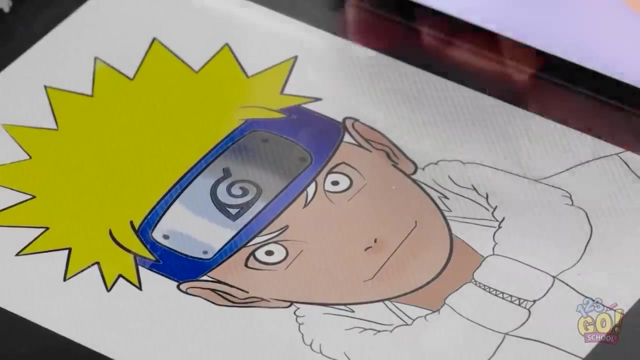 It's so effective, I'll use blue for the eyes. It's so effective, I'll use a light pink for the skin. Then I'll add darker pink under the nose and on ears. Using the iPad makes it so much easier to give my drawings texture and realism. 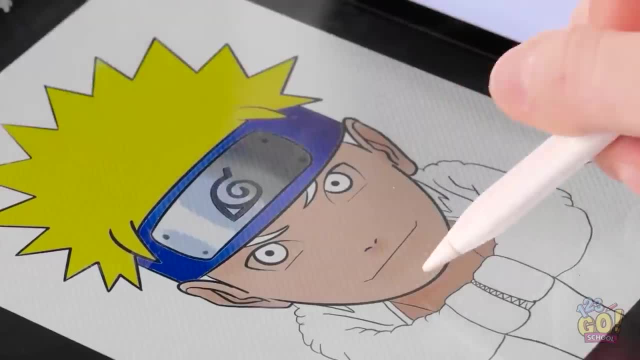 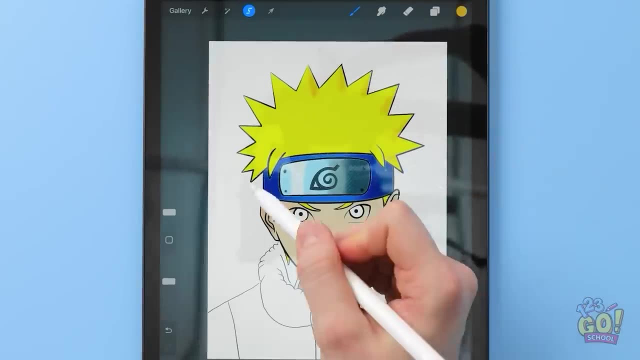 It's just finding the spots where the light falls, Then choosing different tones. I'll use a darker shade of pink on the neck. This would be in shadow. I'll add more details to the hair. It makes his hair look spiked. Now I'll zoom in on his eyes. 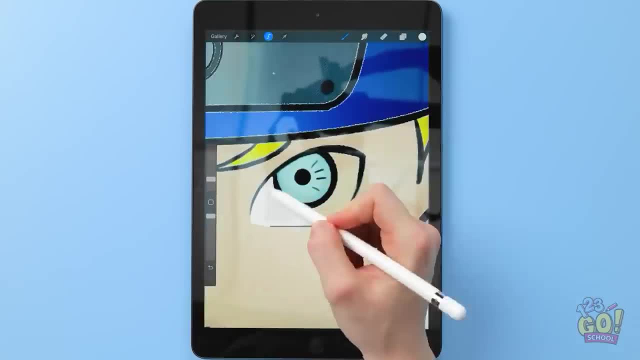 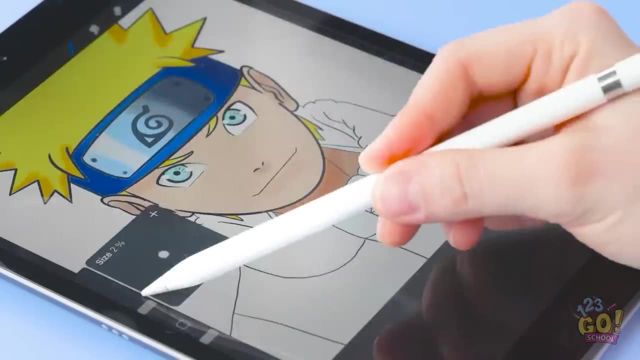 He'll be a blue-eyed boy. I'll add black lines on it. Now I'll select the cutting tool. I'll carefully go around the eyes and the eyelids, Then I'll remove the color. What's next? I know the clothes.